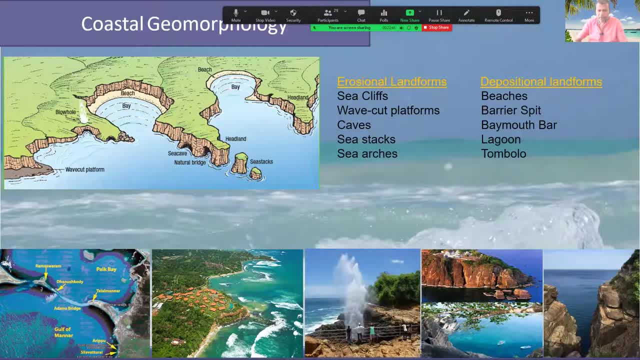 We were discussing a little bit of what kind of coastal structures we can see in the coastal zone. Some of the things that we could see- we already experienced something like this- The connections between the neighboring countries, like here, the Adams Bridge, the shallow areas. 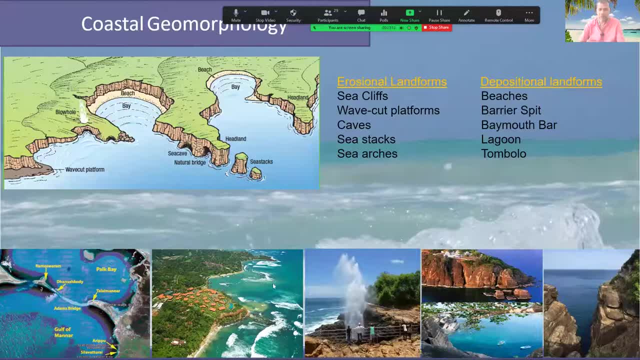 and the bays and lagoons and this kind of a headlands, something coming into the sea. It's unique and very attractive places like there are many headlands like here and the blowholes like in Humana, some of the cliffs, like here in Trincomalee. 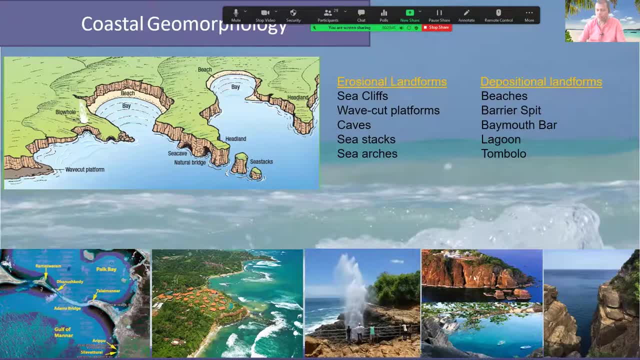 near the cove and the same right here. Likewise, there are many coastal structures. These structures actually are formed due to two different processes. One of the processes we call erosional landforms. Some of these landforms are formed because of the erosional process. 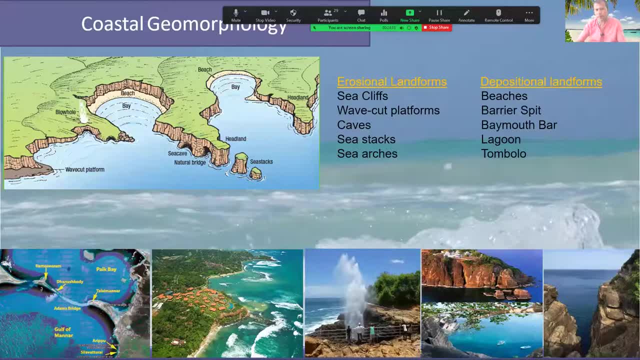 On the other hand, some of the landforms are depositional. These landforms are formed because of the erosional process: The erosional structures versus the depositional structures, For example, the erosional structures of the landforms. Examples are the sea cliffs, something like these cliffs. 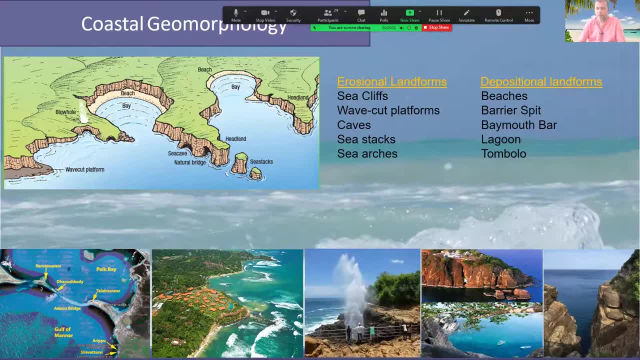 What do you see in Trincomalee? What do you see in Trincomalee? They are erosional. They are not erosional. There are something called the wave cut platforms. It's not very prominent here, but in this top left. 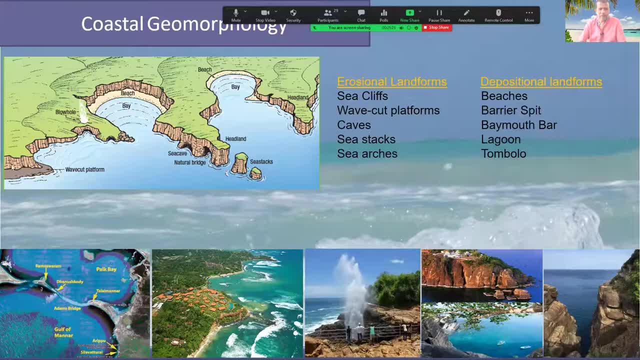 you can see something like here: some platforms, some areas. All these are erosional features, The sea steps, the caves and the sea arcs like here, The natural bridge here, but there is the sea arc here, And the depositional landforms are the beaches, the speed. 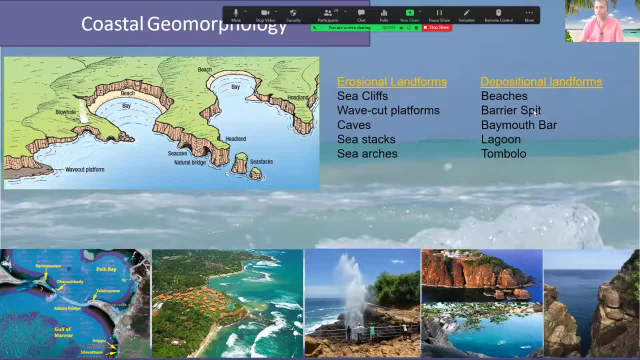 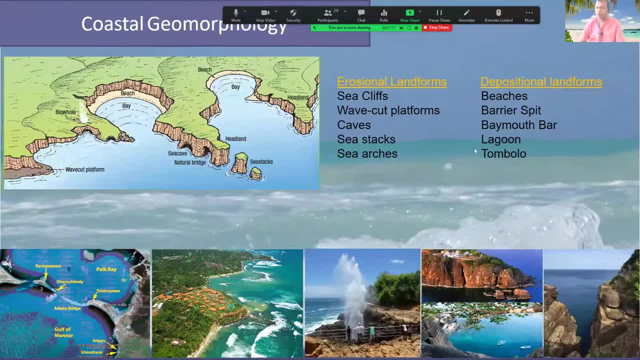 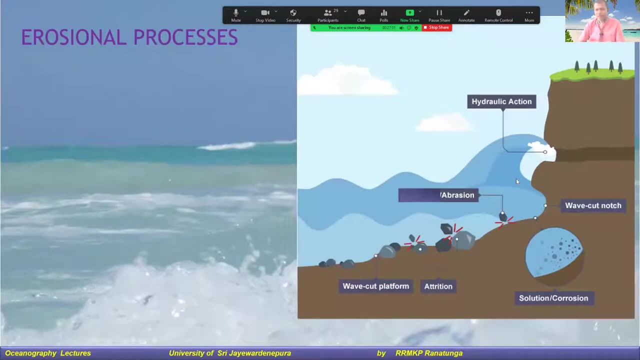 Then a lagoon, Then we have tombolo. I'm pretty sure you haven't heard about this term called tombolo. Let me show you what it is. It's like an abyss. You know what I mean. It's like a small town. 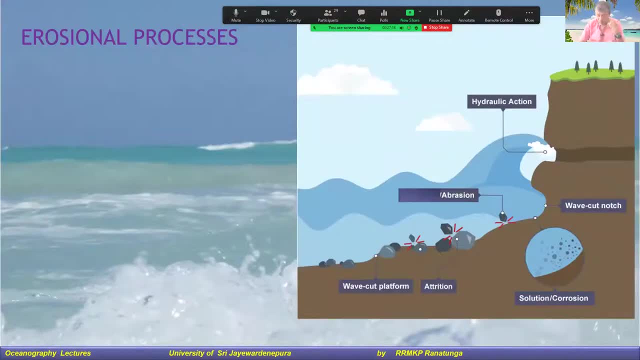 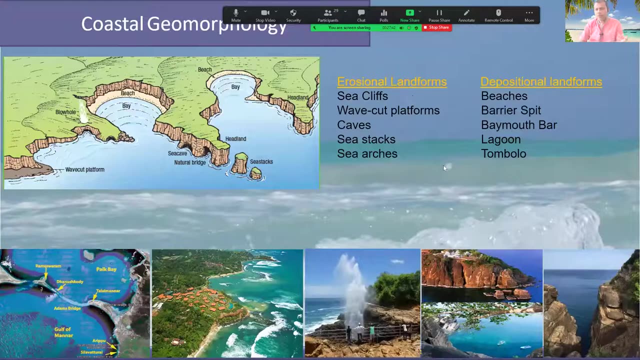 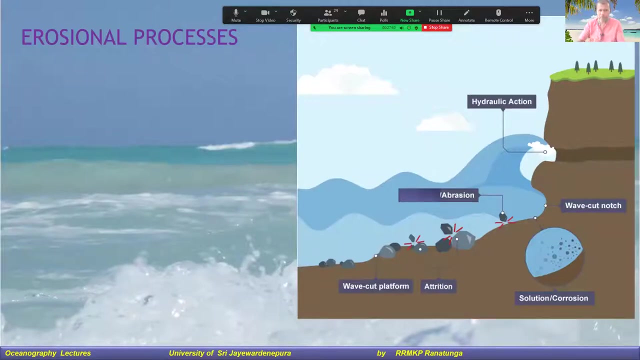 What are these structures? Right Before going into these different structures, this erosional, depositional, as well as there are some coastal processes, There are some erosional processes And these erosional processes cause these different types of erosion In the coastal zone. there are few of these kinds of erosional processes. 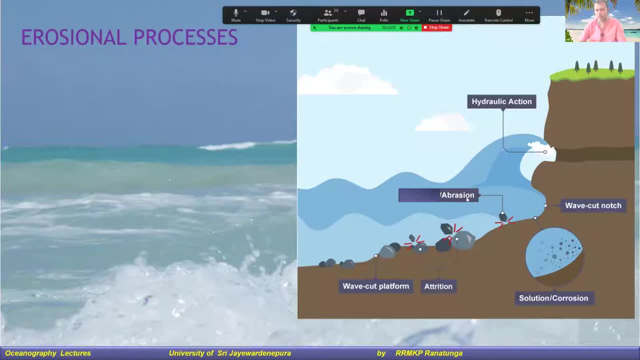 One of such erosional processes is called the abrasion. Let me show you. This is called abrasion, Hydraulic action here. Hydraulic action, This is called abrasion, This is called attrition, This is called solution, This is called corrosion. 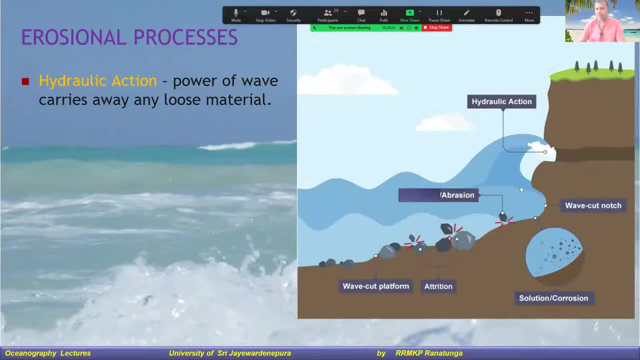 This is called abrasion, We can think of it this way, But something very simple. Hydraulic action means that Hydraulic means water. Water contains power. It can cause erosion. Power of wave carries away loose material, Just like you turn the waves like this for a while. 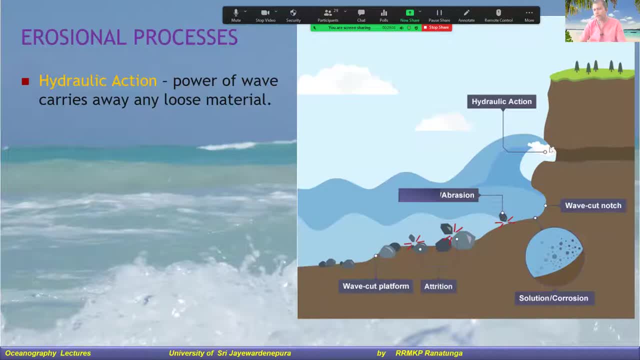 You turn the waves like this for a while. This is called a clip. The second one is the abrasion. Abrasion means particles that are formed by waves. We can call it rocks. Small ones like this are formed by rocks. We can put them together and break them into pieces. 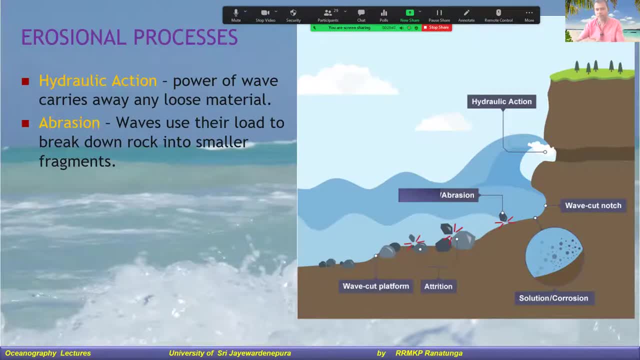 We call it abrasion. This is also because there are no waves. The third type is solute. This is called diffusion, This is called seawater. This is a solvent. Some things can be dissolved. There are structures like calcium carbonate. 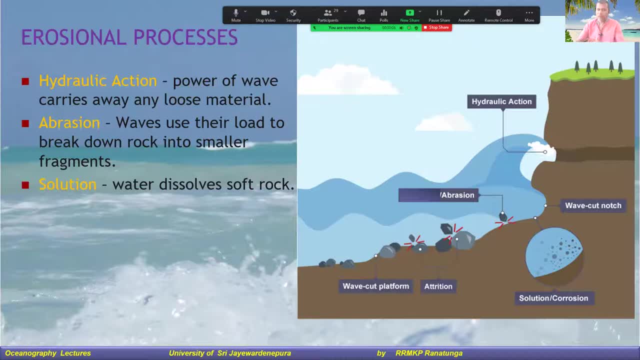 These things can be dissolved in seawater, So it can be dissolved in things like soft rocks. The third type is attrition. This is called attrition. This is different from abrasion and attrition. Abrasion means particles that are formed by waves. 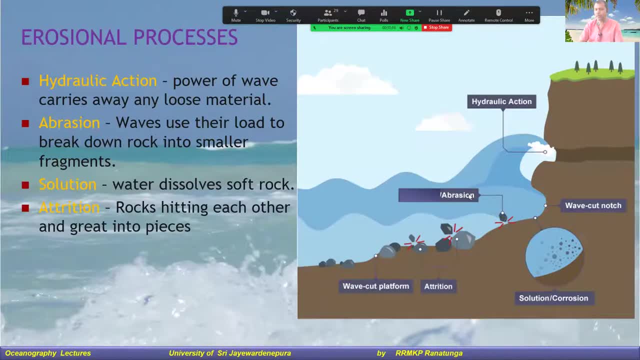 These can be dissolved. This is called attrition. This is called rocks. These are formed by rocks. Particles are formed by rocks. These can be dissolved. These can be dissolved in things like salt. This is called attrition. This is called attrition. 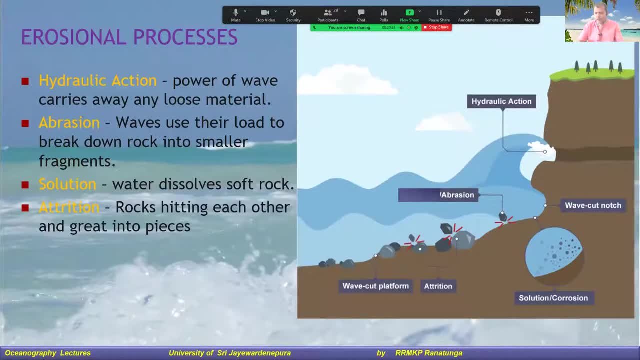 If you have any doubt, you can write down. There is no big thing. This is called attrition, This is called abrasion, This is hydraulic action. This is called solution. This process is called the erosional activities. The reason is because of the coastal zone. 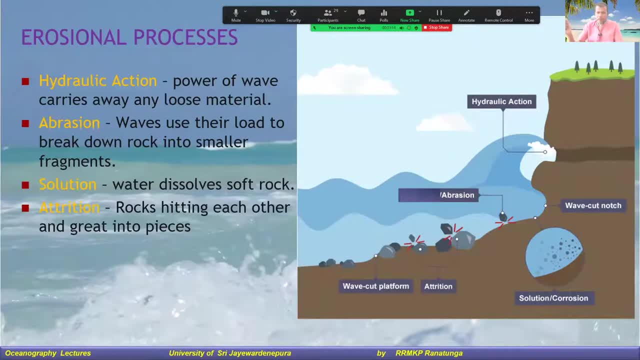 You can find this in other places. we can go to the coastal zone Right, If we know that we can do it for some people. for some people, this is compressed air because it is trapped. It can be trapped in the air. 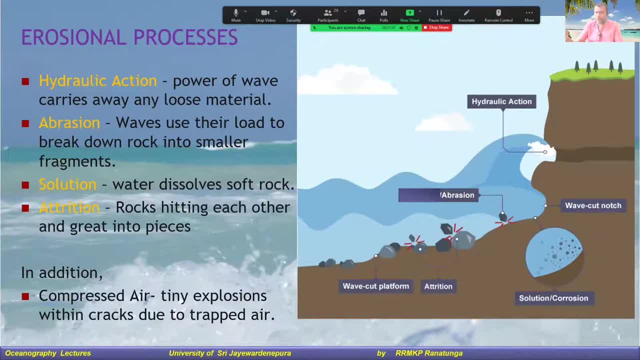 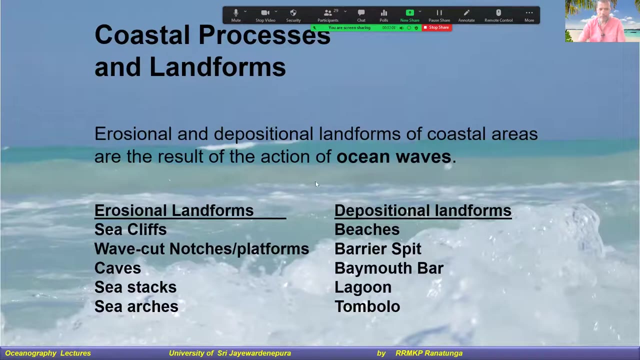 and it can also be removed from the air as it is, but it is very rare. But basically, these are the four forms of erosion that we have seen in the past, So we can say that these are the four forms of erosional courses later on. 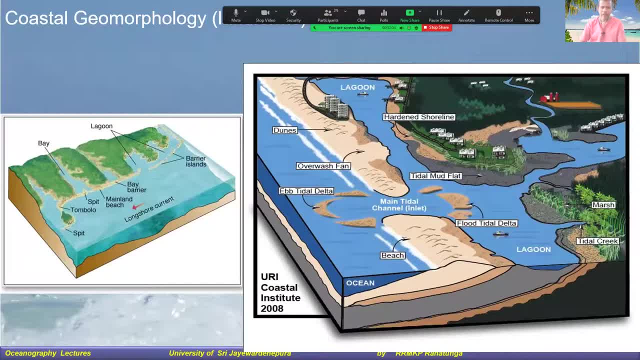 Right. So if you look at the different landforms as you can see here, previously we saw a lot of erosional features, but here you see, most of the structures are actually depositional. So what is depositing here is the sand. 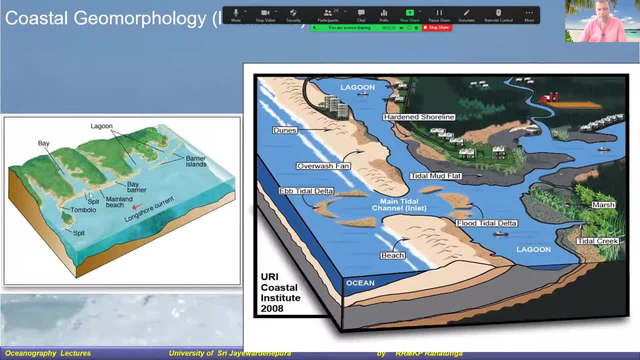 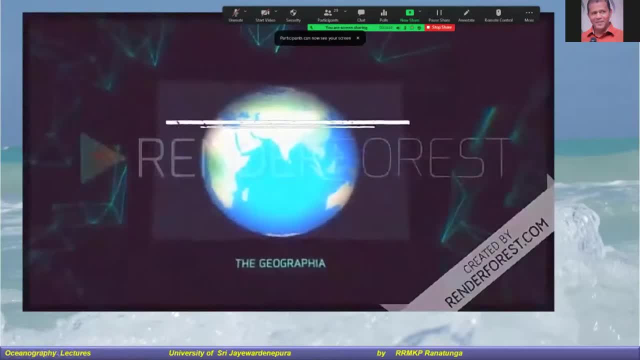 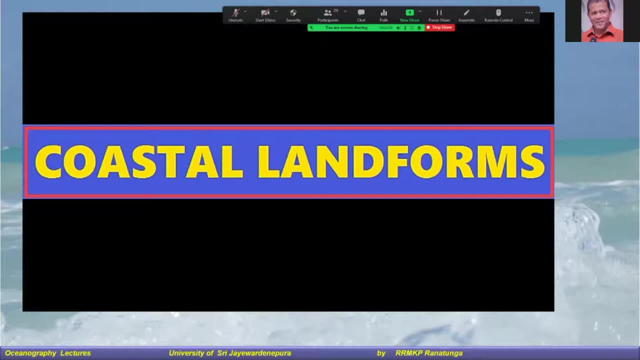 Right. Most of these structures that you can see is because of the sand deposit. Right You can see here is spit Coastal landforms- any of the relief features present along any coast, the result of a combination of processes, sediments and the geology. 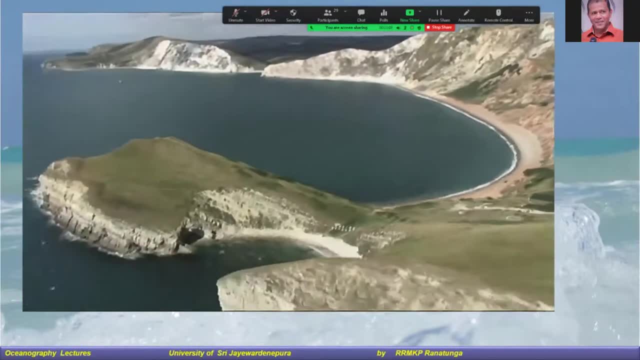 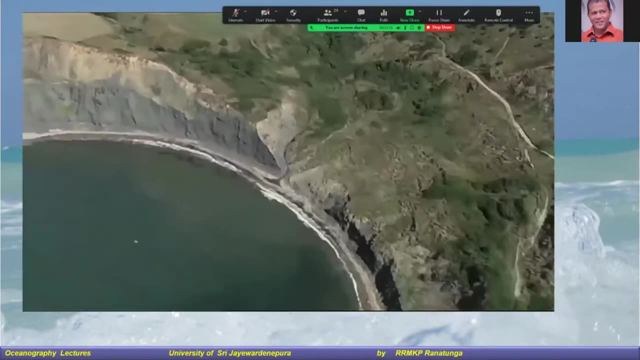 of the coast itself. The coastal environment of the world is made up of a wide variety of landforms, manifested in a spectrum of sizes and shapes ranging from gently sloping beaches to high cliffs. Yet coastal landforms are best considered in two broad categories. 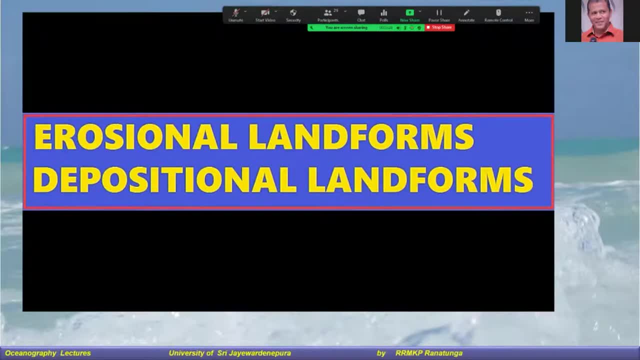 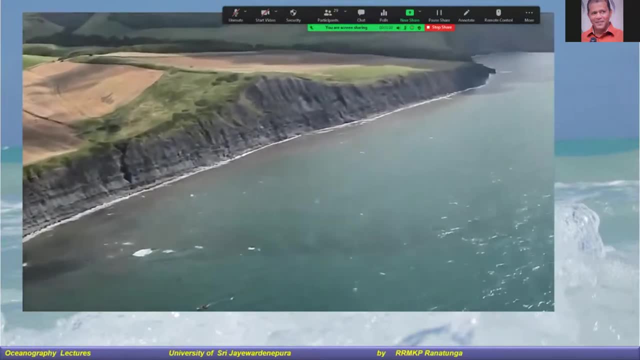 erosional and depositional. In fact, the overall nature of any coast may be described in terms of one or the other of these categories. It should be noted, however, that each of the two major landform types may occur on any given reach of coast. 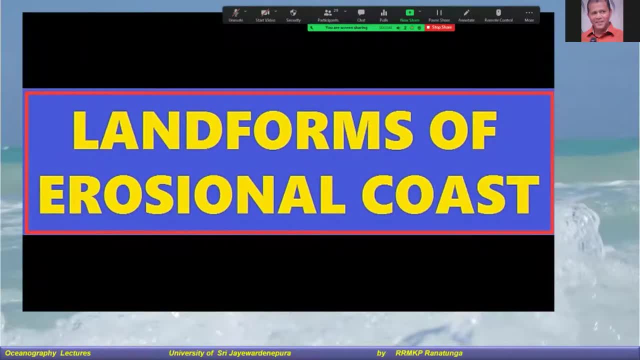 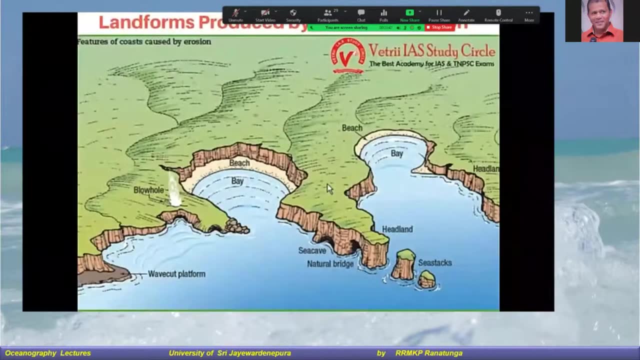 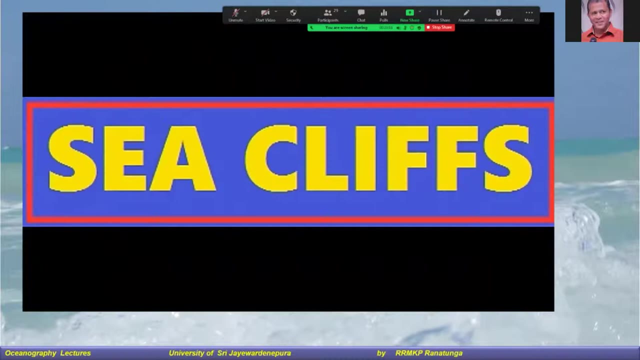 Landforms of erosional coasts. There are two major types of coastal morphology. one is dominated by erosion and the other by deposition. They exhibit distinctly different landforms, though each type may contain some features. of the other Seacliffs, The most widespread landforms. 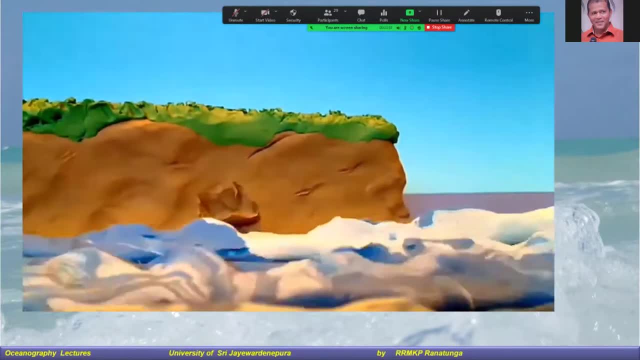 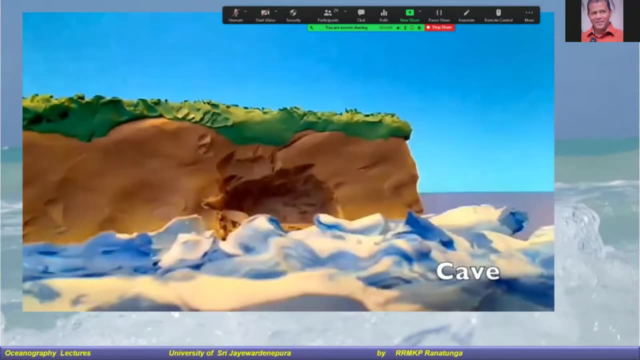 of erosional coasts are sea cliffs. These very steep to vertical bedrock cliffs range from only a few meters high to hundreds of meters above sea level. Their vertical nature is the result of wave-induced erosion near sea level and the subsequent collapse of rocks. 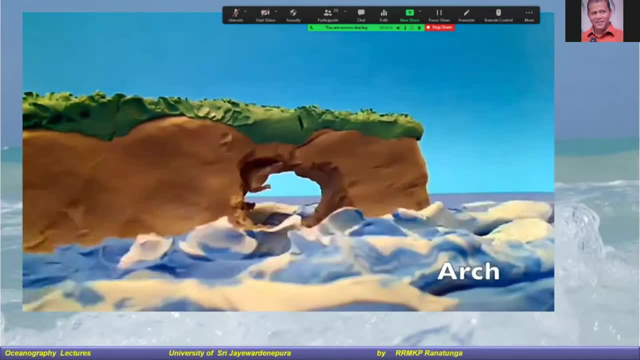 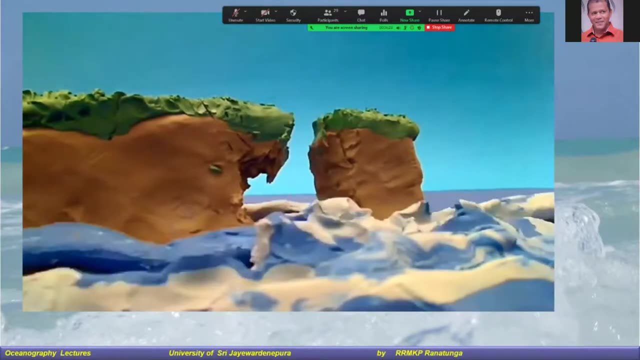 at higher elevation. Cliffs that extend to the shoreline commonly have a notch cut into them where waves have battered the bedrock surface. At many coastal locations, there is a thin, narrow veneer of sediment forming a beach along the base of sea cliffs. This sediment 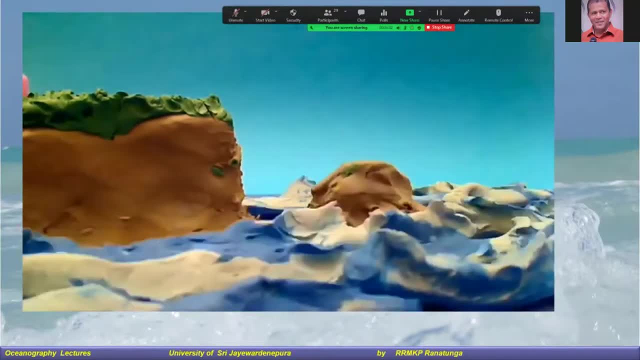 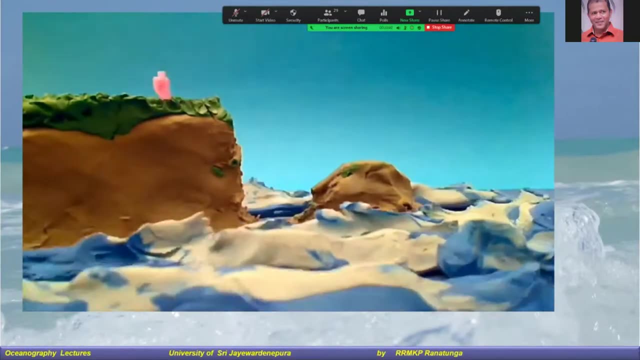 may consist of sand, but it is more commonly composed of coarse material, cobbles or boulders. Beaches of this kind usually accumulate during relatively low wave energy conditions and are removed during the stormy season, when waves are larger. The coasts 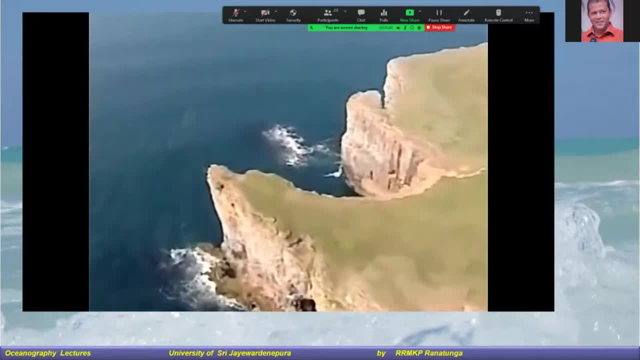 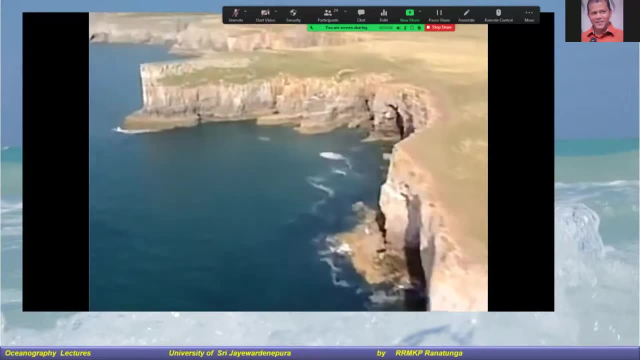 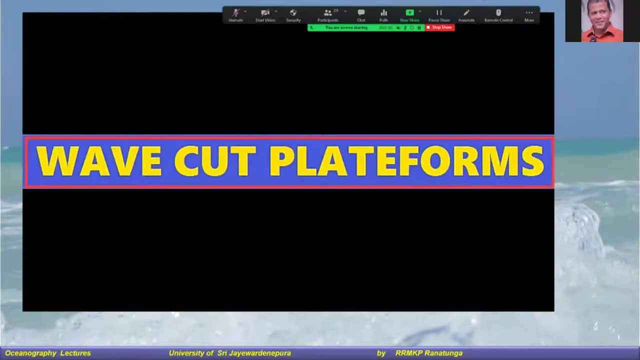 of California and Oregon contain many places where this situation prevails. The presence of even an arrow beach along a rocky coast provides the cliffs protection against direct wave attack and slows the rate of erosion Wave Cut Platforms. At the base of most cliffs along a rocky coast, one finds 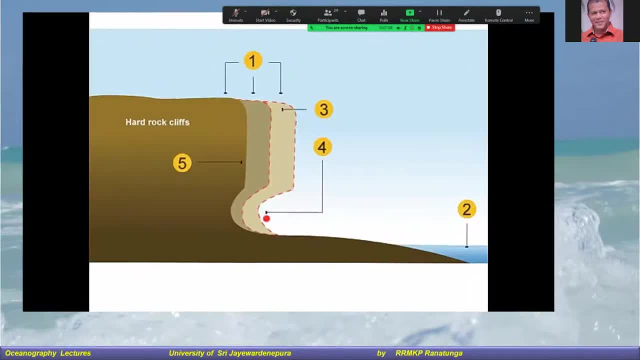 a flat surface at about a mid-tide elevation. This is a bench-like feature called a wave cut platform or a wave cut bench. Such surfaces may measure from a few meters to hundreds of meters wide and extend to the base of the adjacent cliff. They are formed by 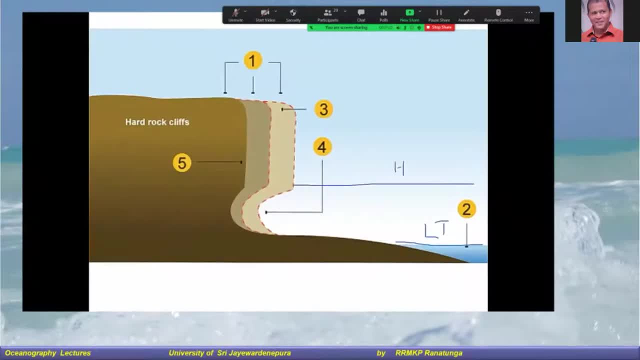 wave action on the bedrock along the coast. The formation process can take a long time depending on the type of rock present. The existence of extensive wave cut platforms thus implies that sea level did not fluctuate during the periods of formation. Multiple platforms of this type. 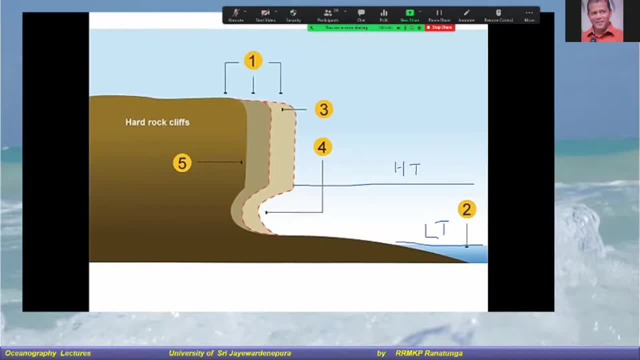 along a given reach of coast indicate various positions of sea level Sea Stacks. Erosion along rocky coasts occurs at various rates and is dependent both on the rock type and on the wave energy at a particular site. As a result of the above-mentioned conditions, 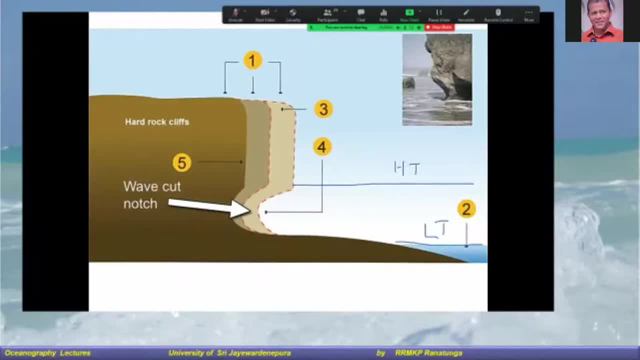 wave cut platforms may be incomplete with erosional remnants on the horizontal wave cut surface. These remnants are called sea stacks and they provide a spectacular type of coastal landform. Some are many meters high and form isolated pinnacles on the otherwise smooth wave cut surface. 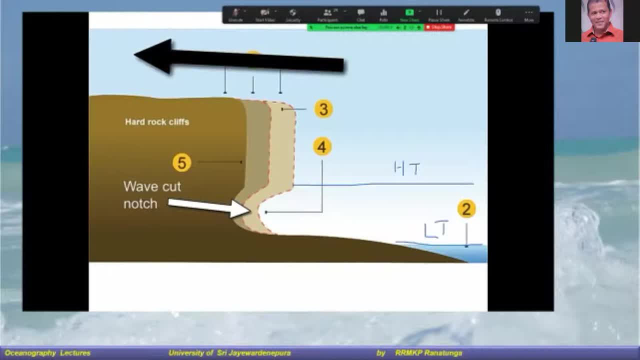 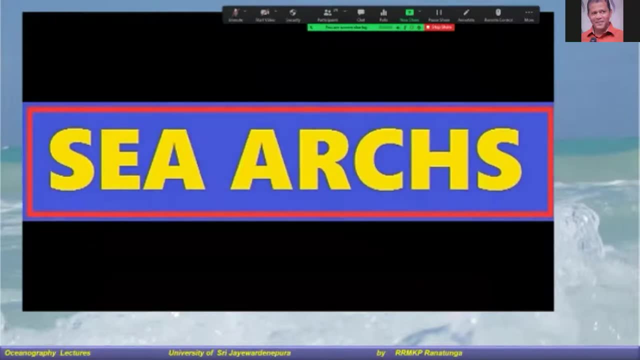 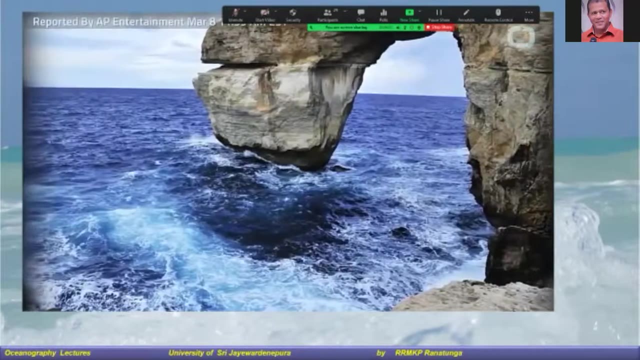 Because erosion is a continual process, these features are not permanent and will eventually be eroded, leaving no trace of their existence. Sea Arches: Another spectacular type of erosional landform is the sea arch, which forms as the result of different rates of erosion, typically due to. 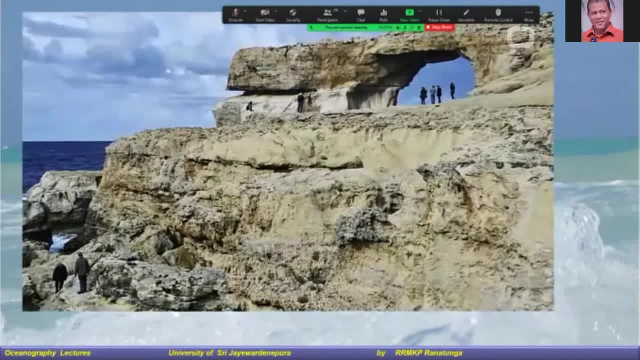 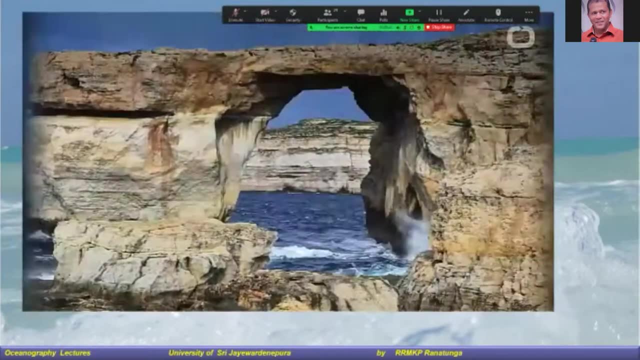 the varied resistance of bedrock. These archways may have an arcuate or rectangular shape, with the opening extending below water level. The height of an arch can be up to tens of meters above sea level. It is common for sea arches to form when 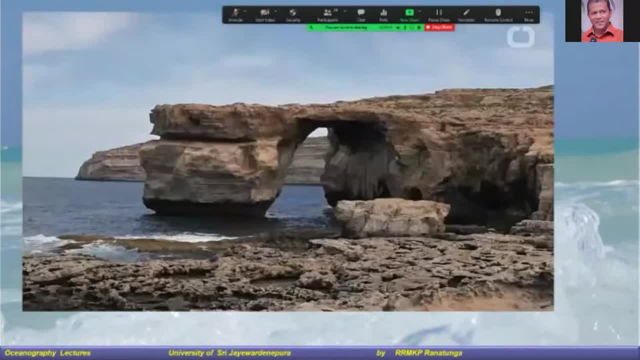 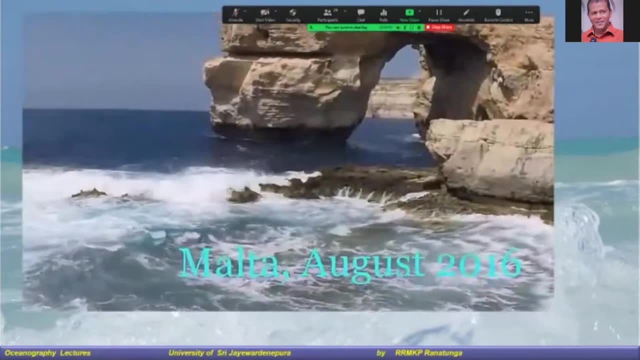 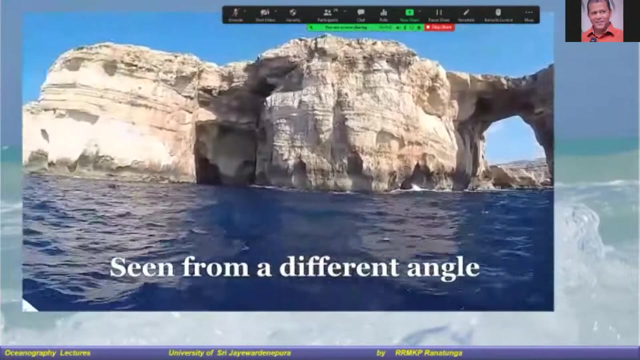 a rocky coast undergoes erosion and a wave cut platform develops. Continued erosion can result in the collapse of an arch, leaving an isolated sea stack on the platform. Still further erosion removes the stack and eventually only the wave cut platform remains adjacent to the 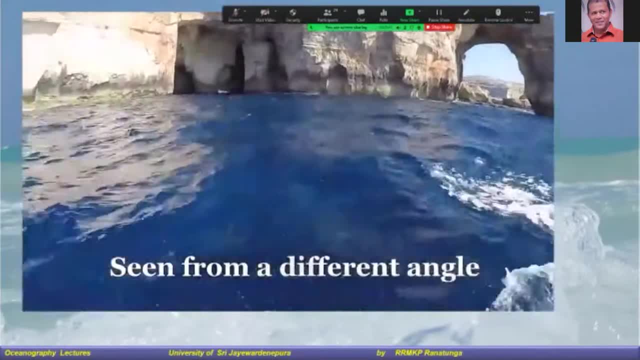 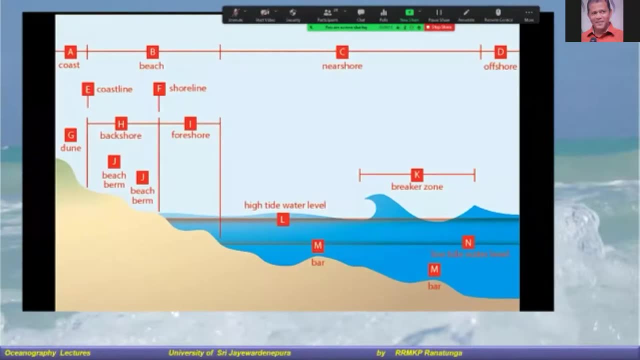 eroding coastal cliff Landforms of Depositional Coasts. Depositional coasts may experience erosion at certain times and places due to such factors as storms, depletion of sediment supply and rising sea level. The latter is a continuing problem, as the mean annual temperature of the 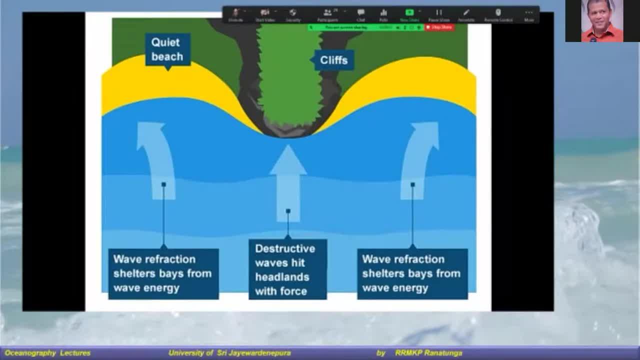 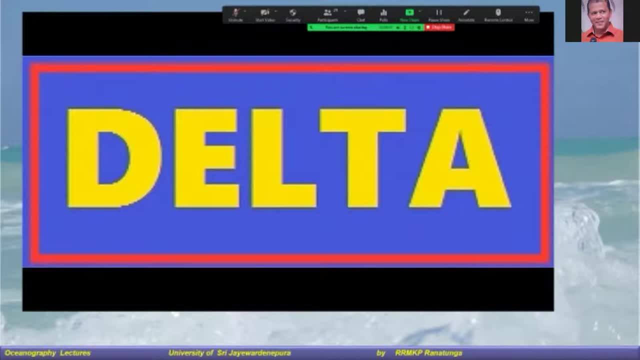 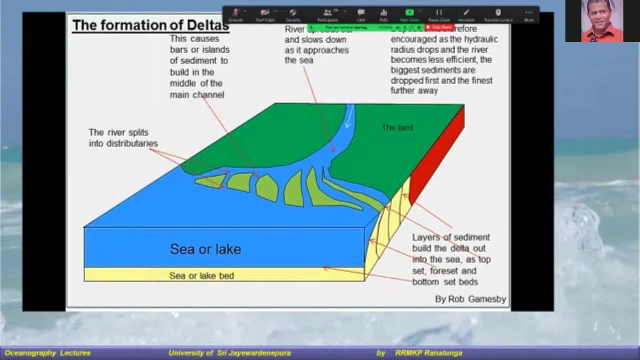 earth rises and the ice caps melt. Nevertheless, the overall long-range tendency along these coasts is that of sediment deposition. Deltas at the mouth of a river extending beyond the trend of the adjacent coast is called a delta. Deltas vary greatly in both size and shape. 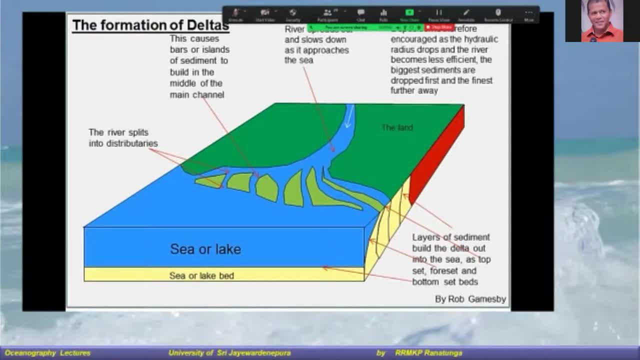 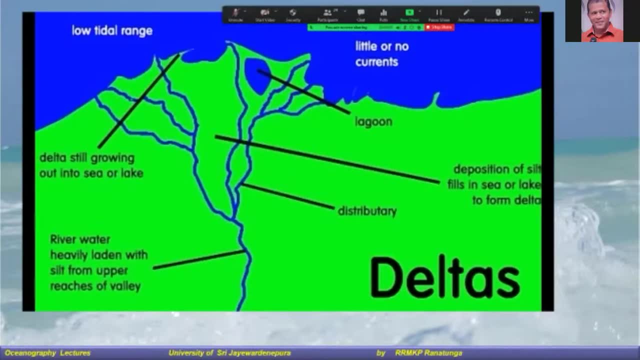 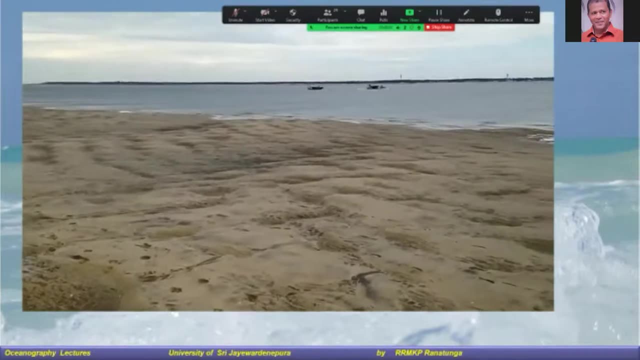 but they all require that more sediment is deposited at the river mouth and can be carried away by coastal processes. A delta also requires a shallow site for accumulation, namely a gently sloping continental shelf. The size of a delta is typically related to the size. 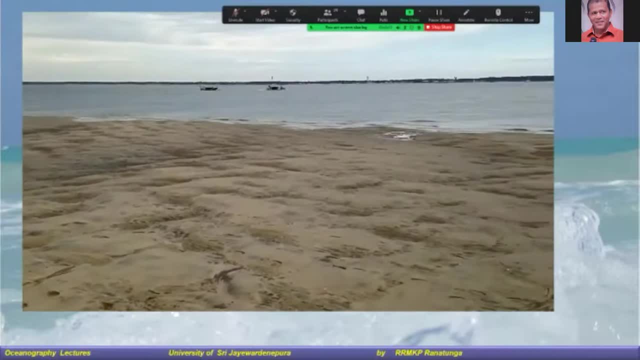 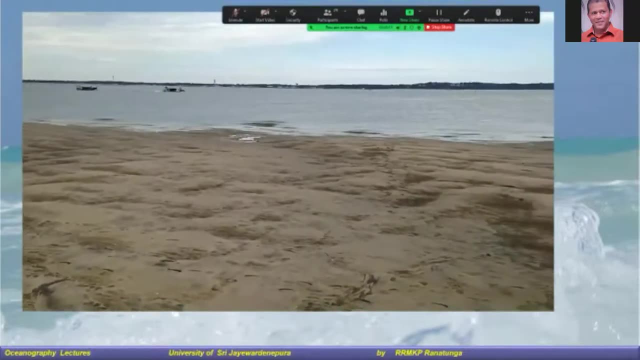 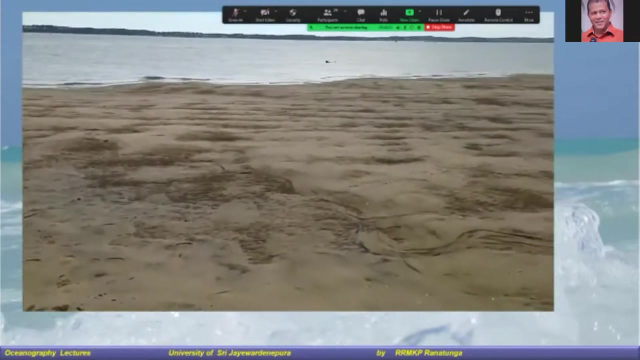 of the river, specifically to its discharge. The shape of a delta, on the other hand, is a result of the interaction of the river with tidal and wave processes along the coast. A classification utilizing each of these three factors as end members provides a good way of considering the variation. 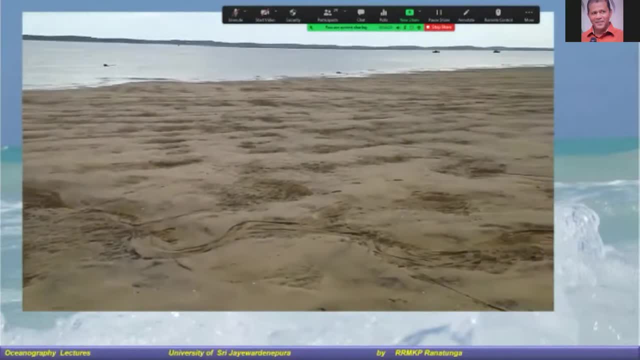 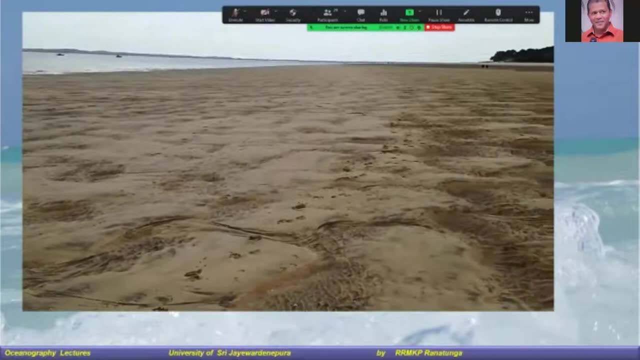 in delta morphology, Figure 1.. River-dominated deltas are those where both wave and tidal current energy on the coast is low and the discharge of water and sediment are little affected by them. The result is an irregularly shaped delta with numerous digitate distributaries. 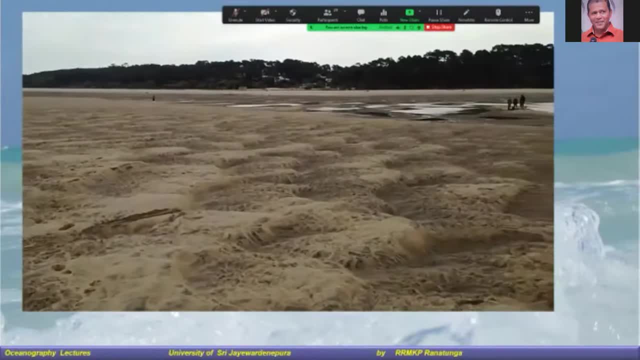 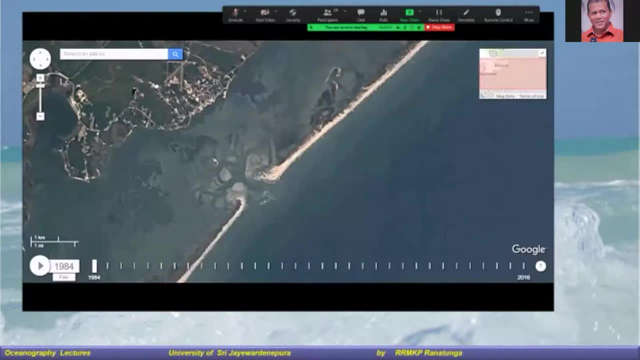 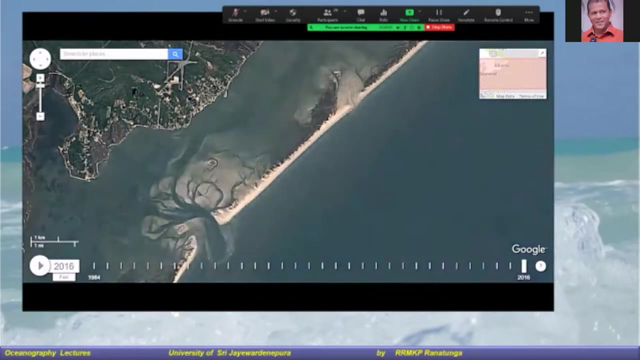 The Mississippi Delta is a good example of a river-dominated delta: Barrier Island. Many depositional coasts display a complex of environments and landforms that typically occur together. Irregular coasts have numerous embayments, many of which are fed by streams. 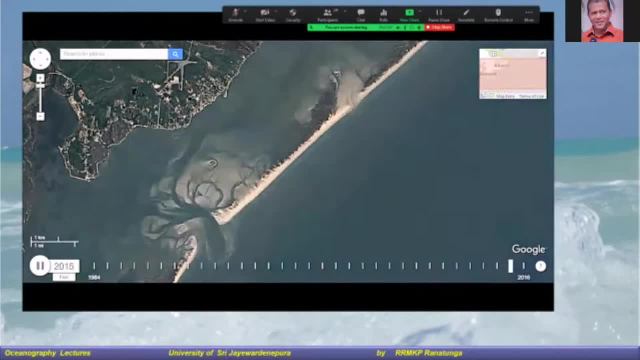 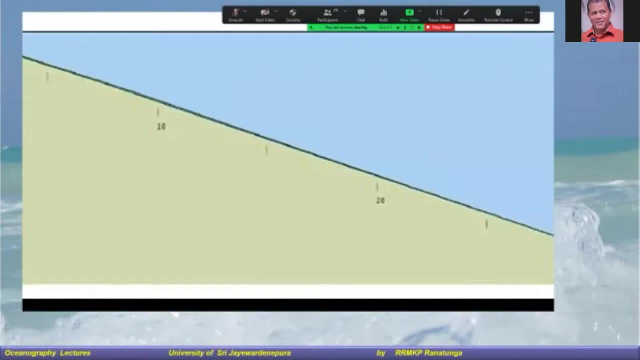 Such embayments are called estuaries and they receive much sediment due to runoff from an adjacent coastal plain. Seaboard of the estuaries are along the shore. The estuaries are located on eight barrier islands that generally parallel the shore, Consisting. 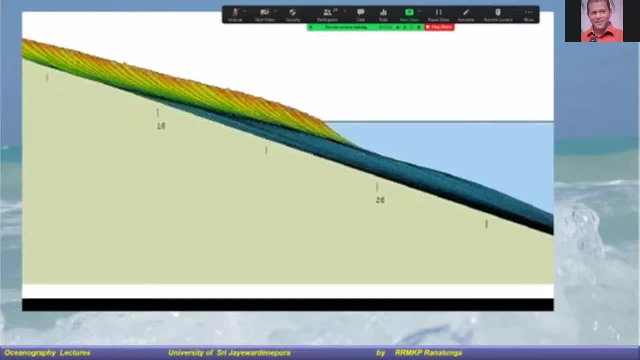 mostly of sand. they are formed primarily by waves and longshore currents. These barrier islands are typically separated from the mainland and may have lagoons, which are long, narrow coastal bodies of water situated between the barrier and the mainland. Most barrier islands contain 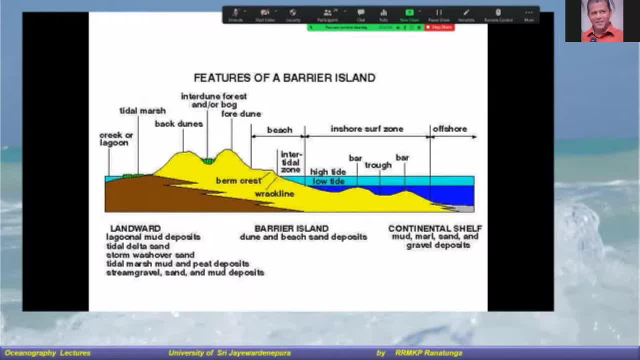 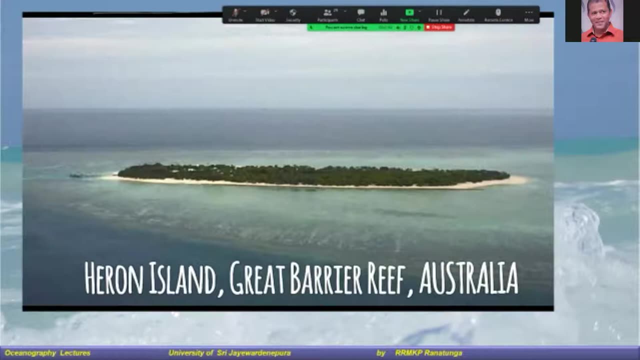 a well-developed beach, coastal dunes and various environments on their landward side, including tidal flats, marshes or wash over fans. Such coastal barriers are typically interrupted by tidal inlets, which provide circulation between the various coastal bays and the open marine environment. 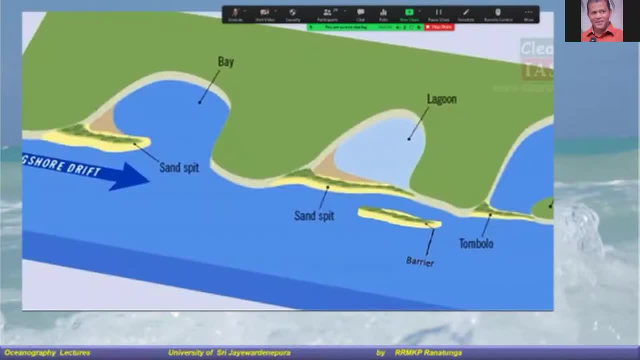 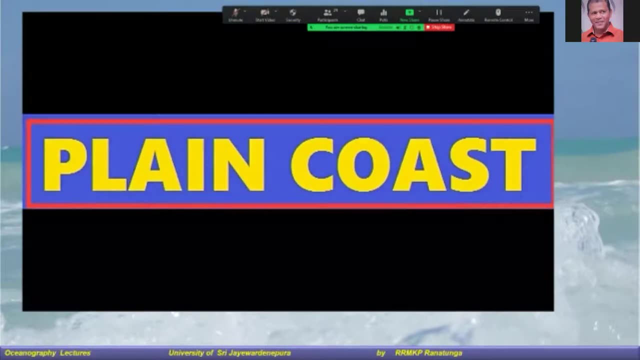 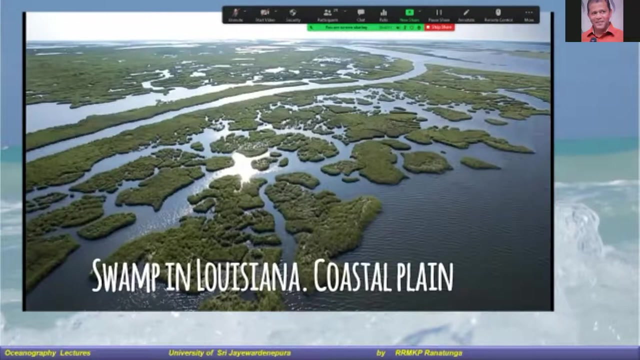 These inlets also are important pathways for organisms that migrate between coastal and open marine areas, as well as for pleasure and commercial boat traffic. Strand Plain Coasts, Some wave-dominated coasts, do not contain estuaries and have no barrier island system. These coasts, however, do have beaches and dunes and may even have coastal marshes. 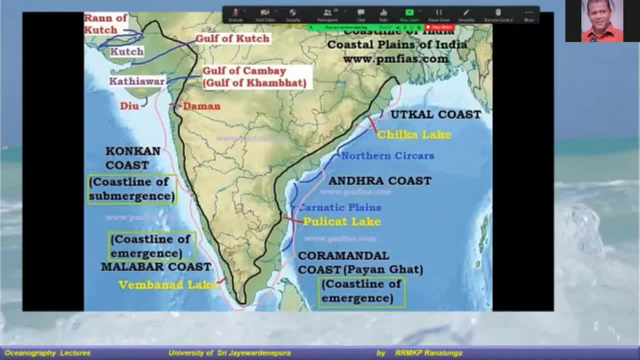 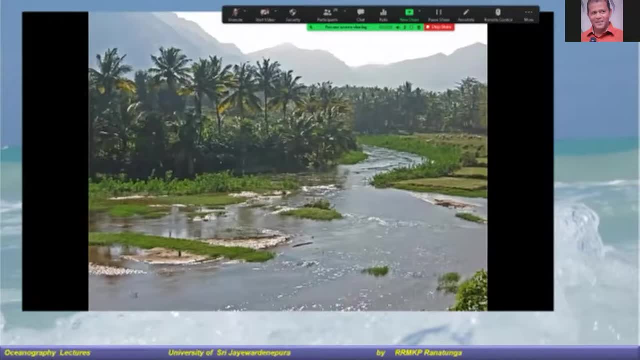 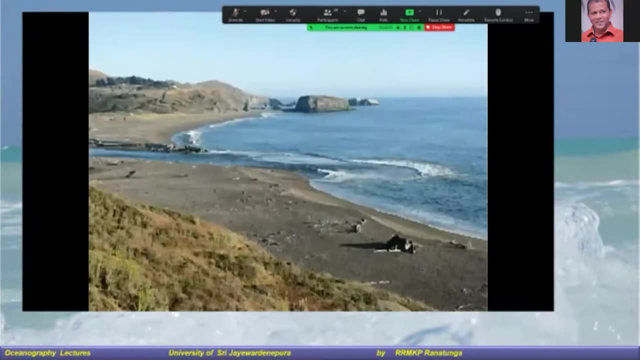 The term strand plain has been applied to coasts of this sort. Examples include parts of western Louisiana and eastern Texas. In most respects they are similar in morphology to barrier islands, but lack inlets, Beaches and Coastal Dunes. There are several specific landforms representative. 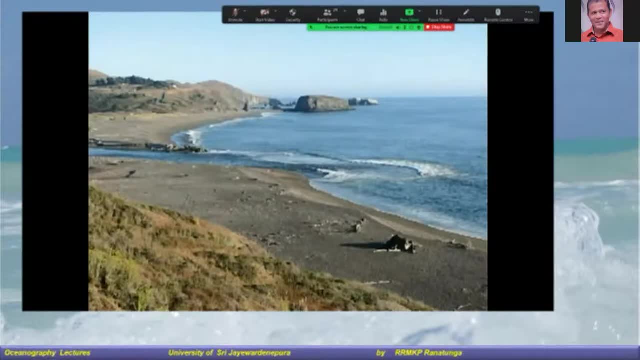 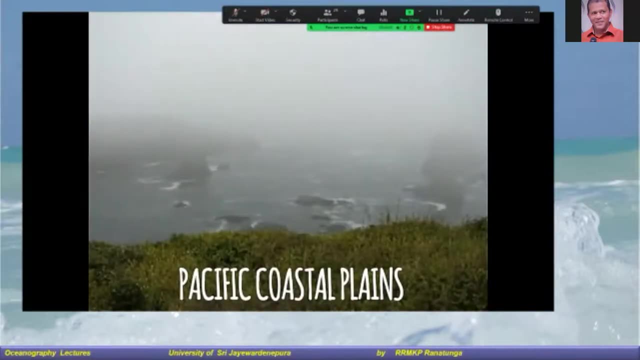 of coastal inlets. There are three major environments that are common to each of the three major categories described above. Especially prominent among these are beaches and dunes. They are the primary landforms on barrier islands, strand plain coasts and many deltas. 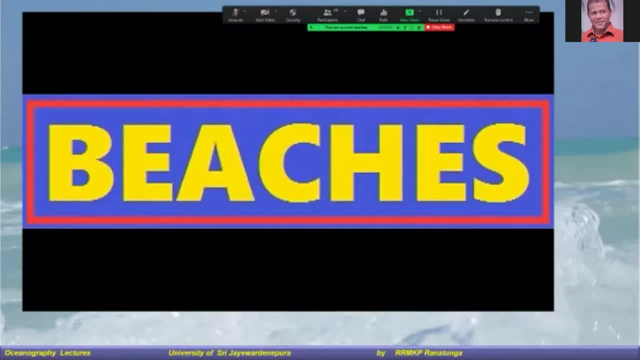 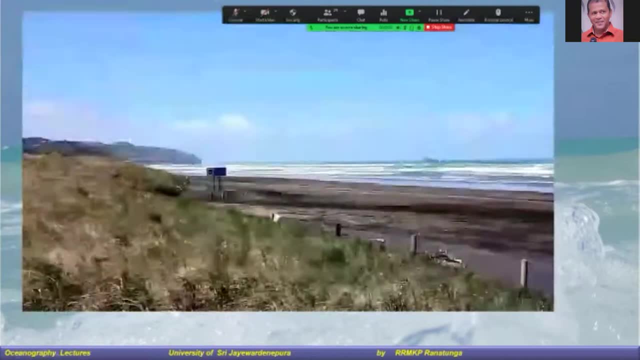 particularly the wave-dominated variety Beaches. A consideration of the beach must also include the seaward-adjacent nearshore environment, because the two are intimately related. The nearshore environment extends from the outer coast to the southern coast. The nearshore environment extends from the outer coast to the southern coast. 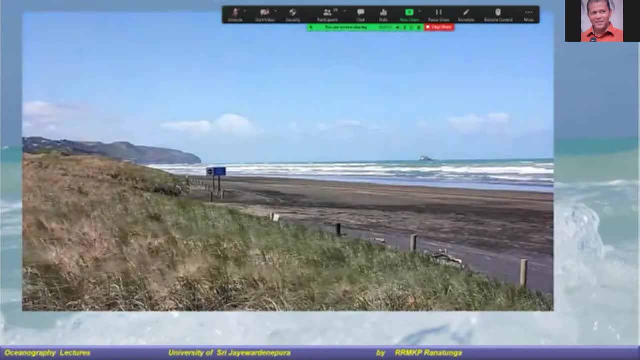 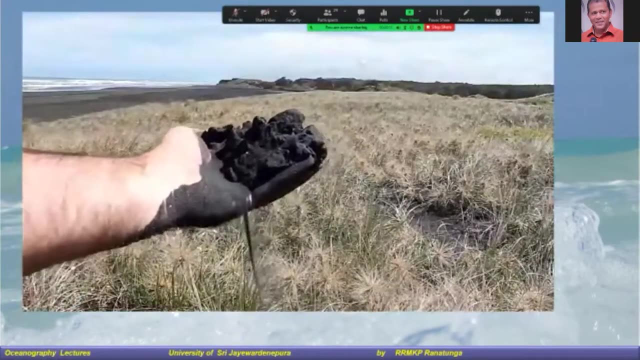 The beach extends from the outer limit of the longshore bars that are usually present to the low tide line. In areas where longshore bars are absent, it can be regarded as coincident with the surf zone. The beach extends from the low tide line to the distinct change in slope and or material. 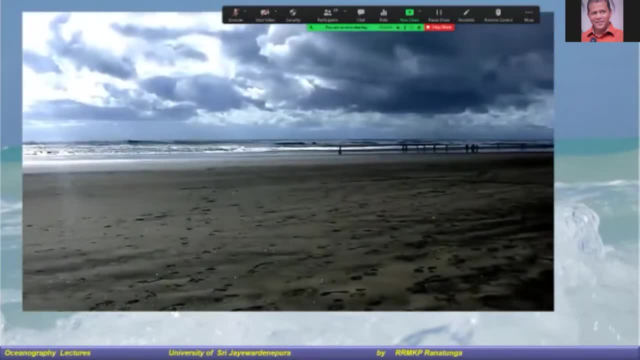 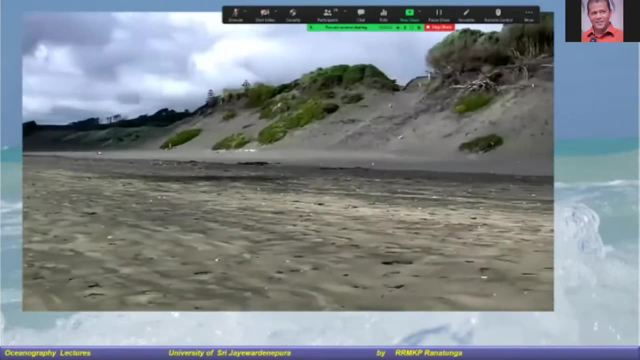 landward of the unvegetated and active zone of sediment accumulation. It may consist of sand, gravel or even mud, though sand is the most common beach material. Coastal Dunes: A mean beach is the most common beach material- Coastal dunes. 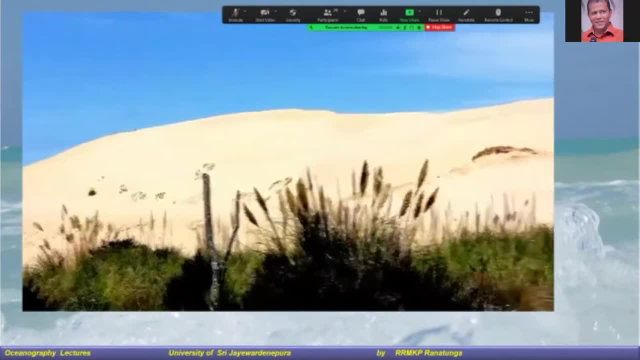 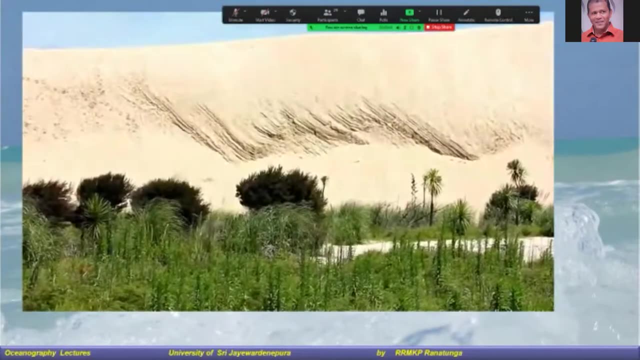 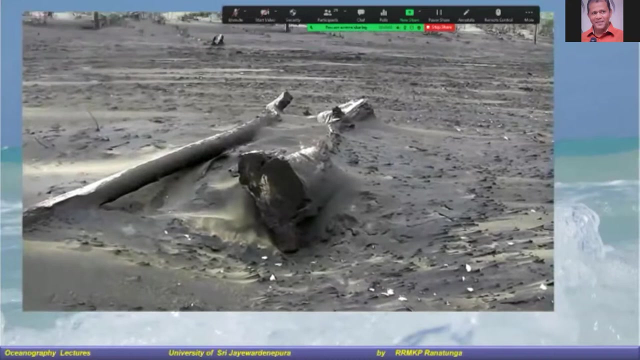 Coastal dunes immediately landward of the beach are commonly found large linear accumulations of sand, known as dunes For coverage of dunes. in arid and semi-arid regions. they form as the wind carries sediment from the beach in a landward direction and deposits it wherever an obstruction hinders. 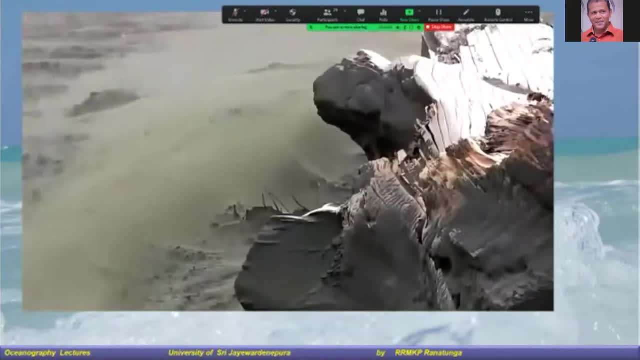 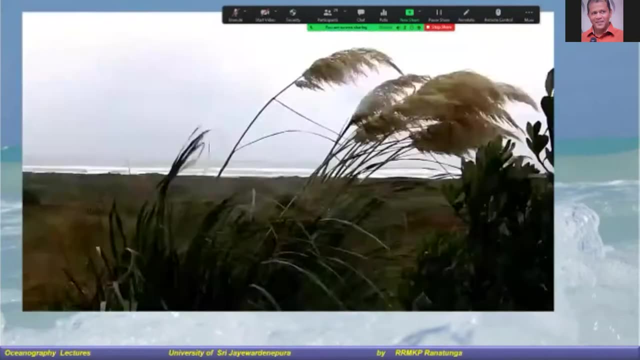 further transport. Sediment supply is the key limiting factor in dune development and is the primary reason why some coastal dunes, such as those on the West Florida Peninsula, are quite small. Coastal dunes are the most common sediment in the region. 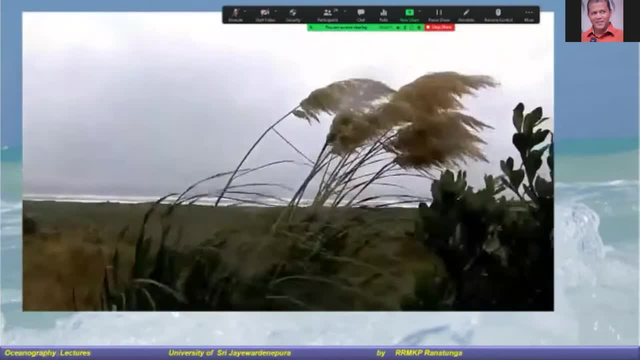 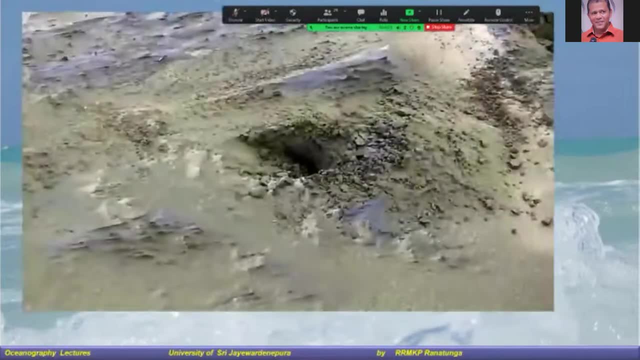 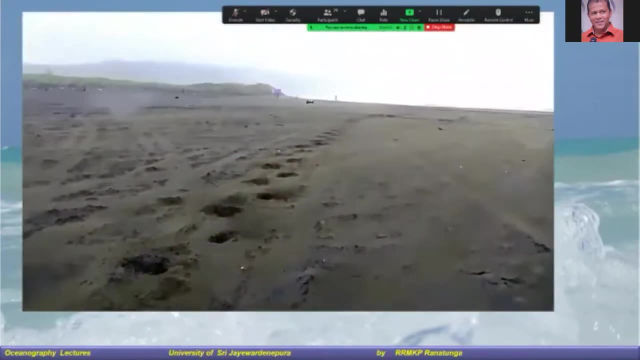 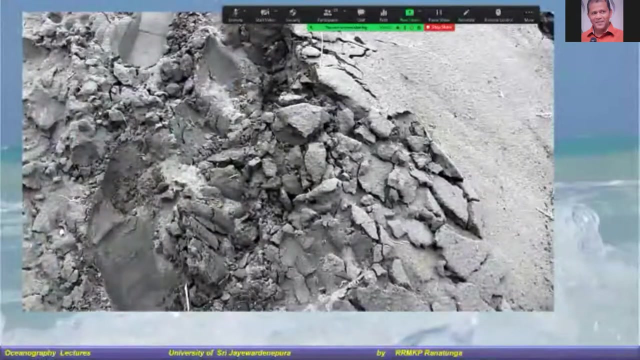 Coastal dunes are the most common sediment in the region. They may not solely contain sediment there, but in many of the most egg-like areas, for example Texas and the context of the Montana expliers, avengers and tartute frifts. and 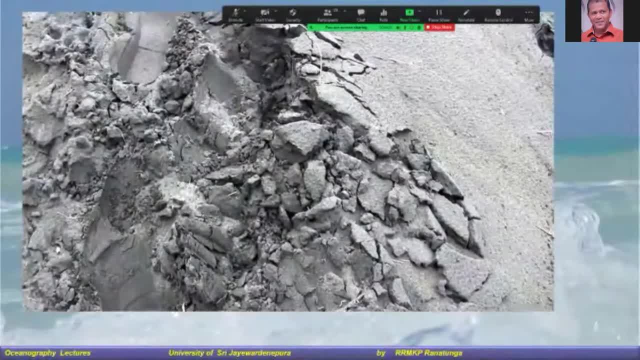 the Hin Man fish. In addition to sand accumulated on the coast, they are also known as salt sandprop sheets, As resources to keep sea catchers ready and maintain gentle Talon. they may also be used as sediment throughout a stream in torrential terrain. 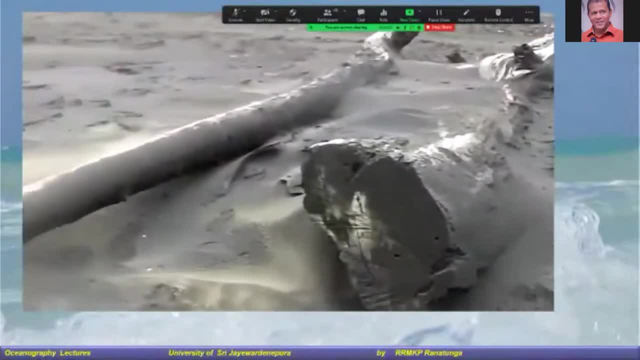 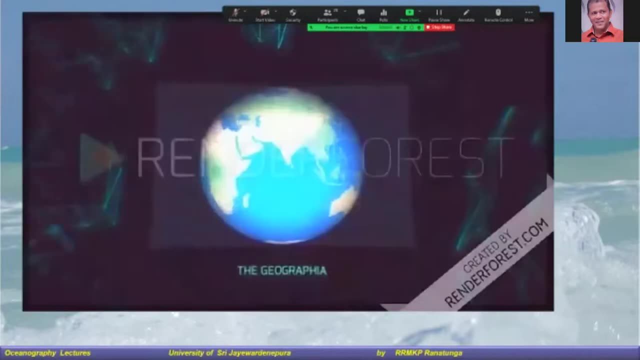 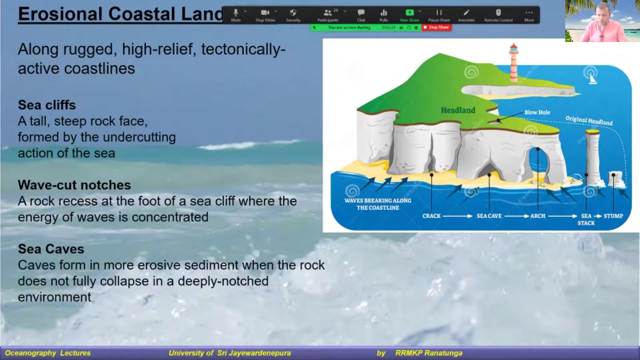 or island or a strand. plain coasts exhibit numerous essentially parallel dune ridges testifying to this type of growth. thank you so much for the watching the. so almost all the structures will talk that we do explain. I'll just very briefly explain what are those. so sea cliffs, of course, as one. 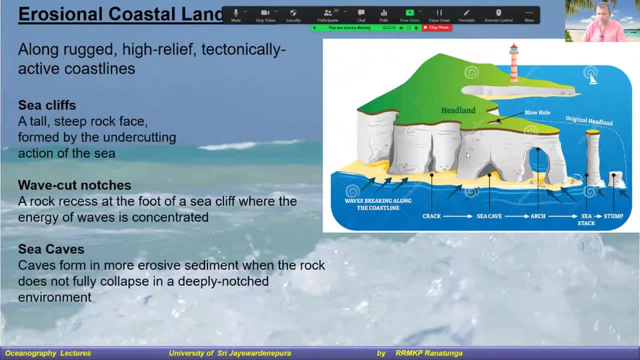 we would see in the Trincomalee. they are very basically, after eroding the, the sand, whatever the rocks can be seen. so these kind of things are the sea cliffs, like the cliff in the Trincomalee is actually also very deep, and then, if any, 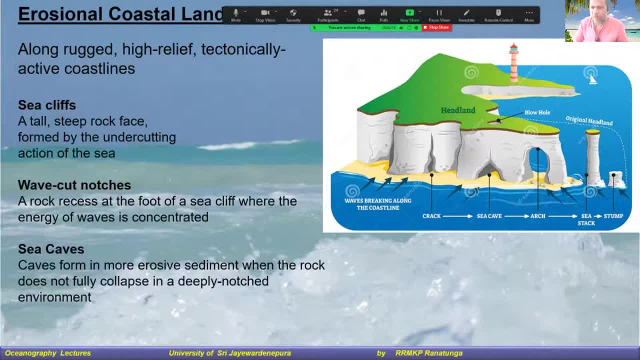 chance you go to Trincomalee, you better now go to that the cove and then from there you can see this beautiful cliff facet, overlooking the Trincomalee Bay, so one of the beautiful scenery to look at. then the wave cut notches are not very common, but you see they like if you look at these. 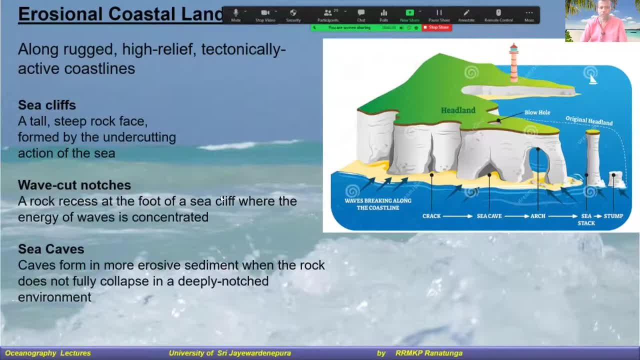 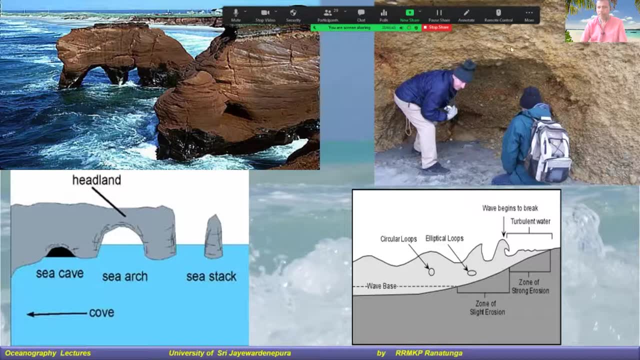 cliffs very carefully, you will see some of these kind of notches and including the caves I like here, the cave actually. this can be later become this kind of an arch right and once the arch is eroded and what is left here is the, the sea stack right once it ordered here. 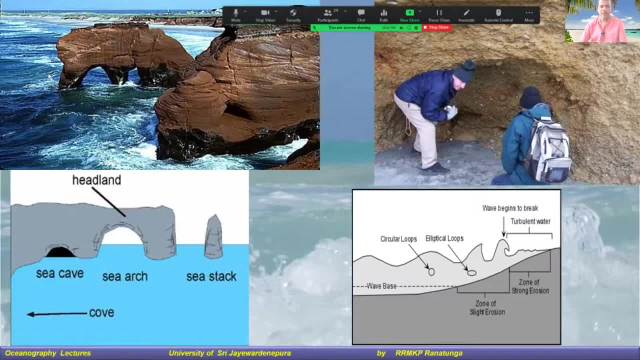 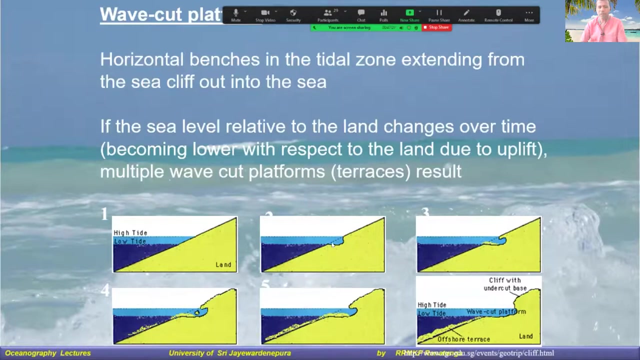 and become a stack, or even here, and if it is severely eroded, then it becomes stump stump stuff like this: based up right, so that's how these are formed. so in the arch and the top that can be a bridge. right, that's how these are formed. in the wave cut platform: so it's. 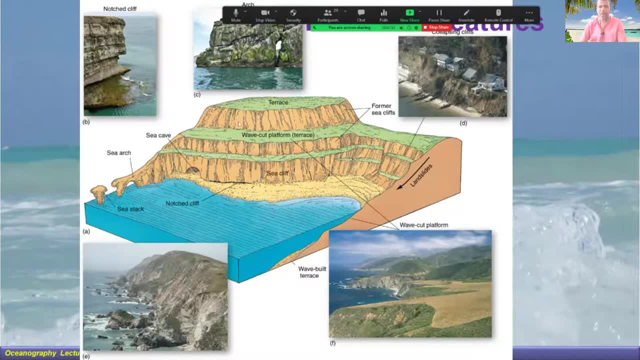 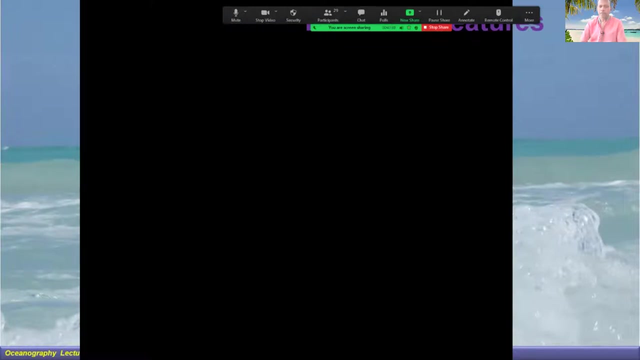 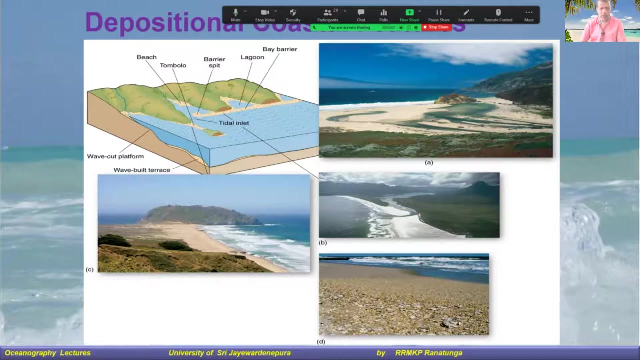 well explained in the videos as well. this is how it would appear, like fused terraces or the platforms right- um, not very common in some, but, uh, but not very prominent right right now. all these are erosional landforms. then the other landforms are erosional landforms. 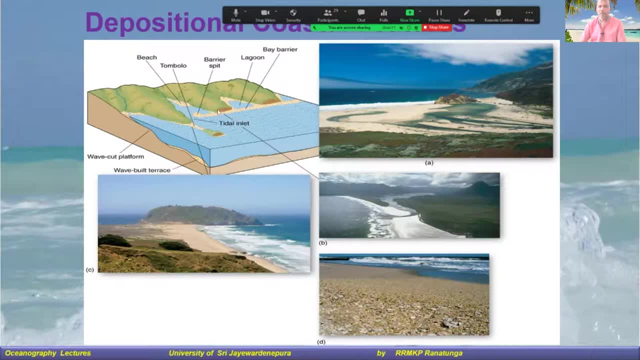 right, something like the spit, or if it is heavily deposited and it is long term, and they can form a arch on the so-called landforms, the arch island right like here, if it is deposited for long period of time and become island, like here, right. so then become a barrier island and they can be a, sometimes a city in some countries. 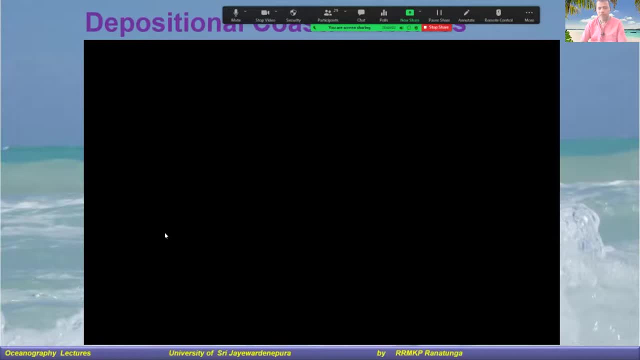 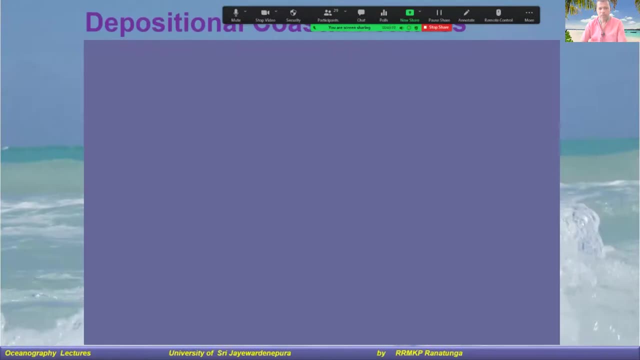 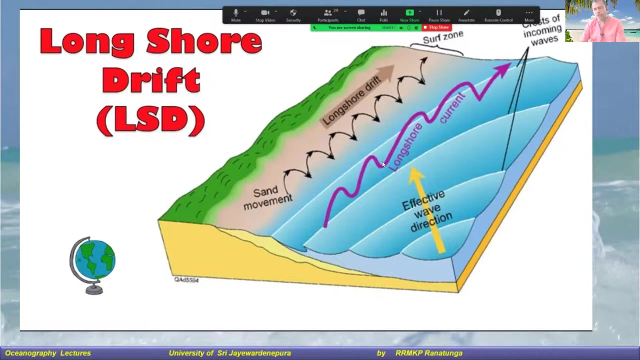 right. so that's, these are the depositional forms, right, uh, now how this, the sand deposition, happened. shallow coastal waters, show currents, long show currents, uh, long show currents have. Now you can experience this if you put a bowl or something like if you throw it in here. 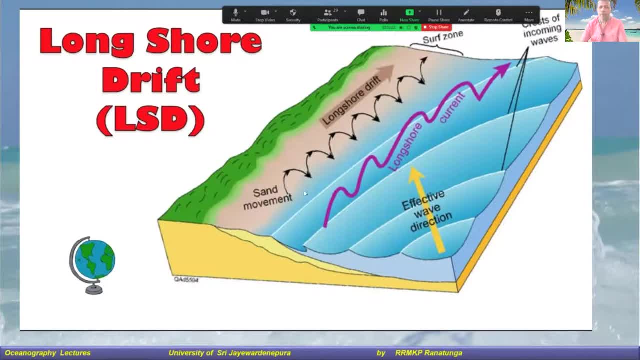 or even a slipper or something. you can see how it moves over the time. Especially if you put a bowl or something like this, you can see how it moves over the time. But if you put a bowl or something like this, you can see how it moves over the time. 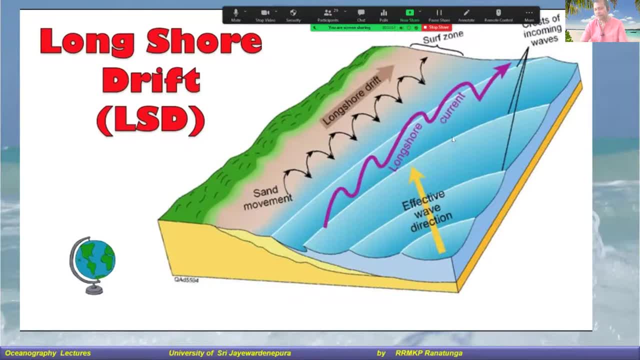 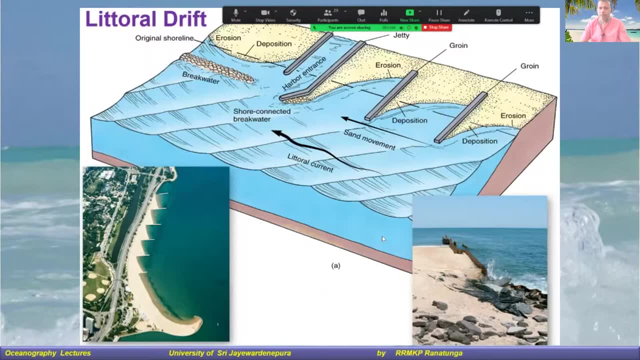 It depends on the currents, direction, the longshore currents. That's how the sediments move in the coast, right, We will talk about this later, just to have an idea. So this Sand, This is how the sand moves and deposits and erodes. 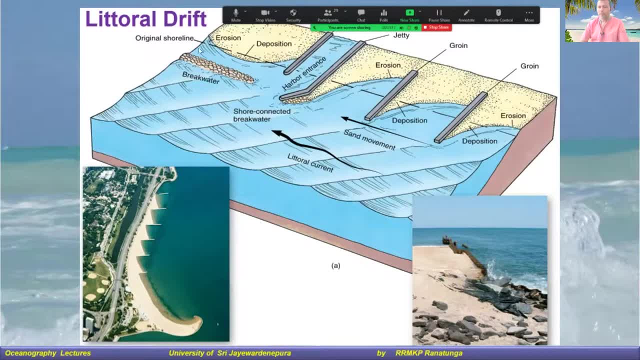 So the sediments are made like this, With barriers made like this. This has a break-quart, especially at the harbor, the port and the entrance. There are break-quart like this And then waves come from side to side and it can get a bit of pressure. 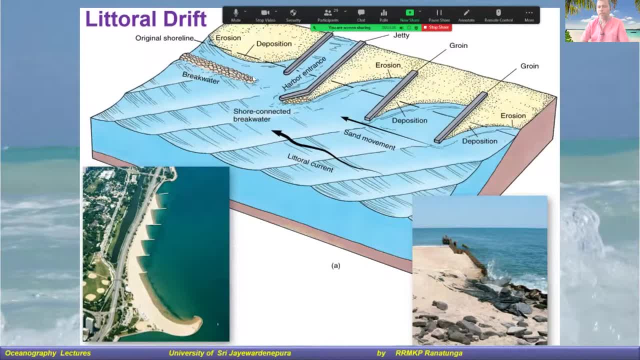 And then waves come from side to side and it can get a bit of pressure On the beach. there is something called a groin In this area. there is a longy and a long curve there. The groin here is used to pull the water down and the water will roll down towards the side. 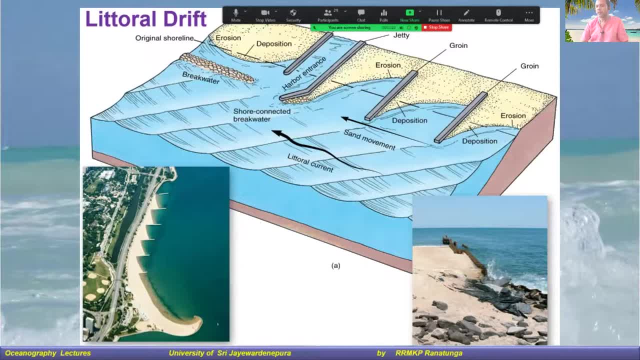 In the case of our current current, as we have a longshore current current here, the grow of the groin will rise and deposit, And this is how the beach was formed: One and a half kilometers, but at the same time the deposit was made. 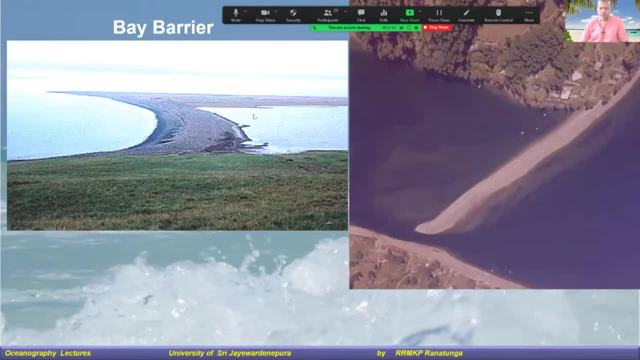 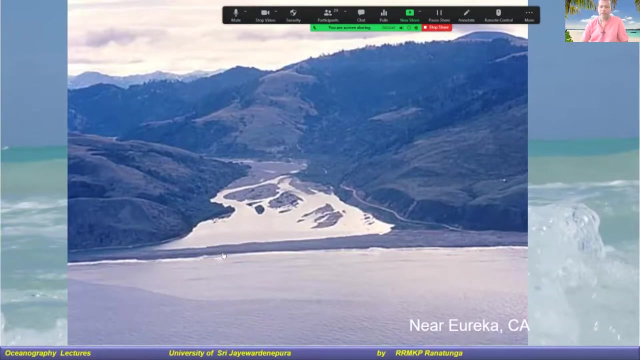 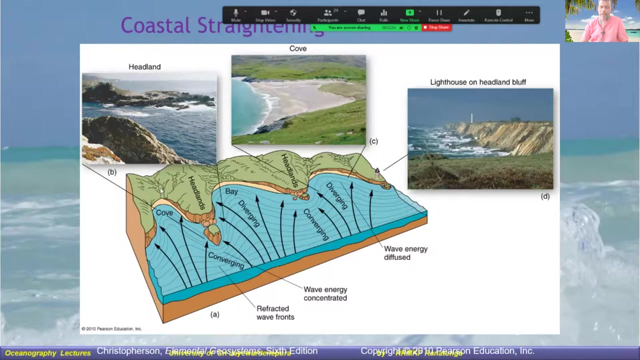 This is a speed, this is a barrier. if it is completely covered, it is not a barrier. it is the same thing. it is a speed, This is a barrier. The other thing is the headlands. If you have a lighthouse, you will see that there are lighthouses everywhere. 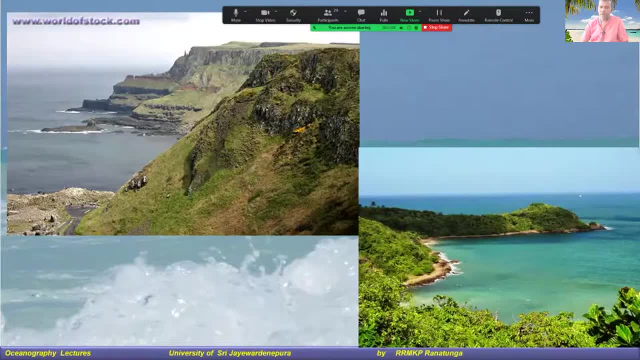 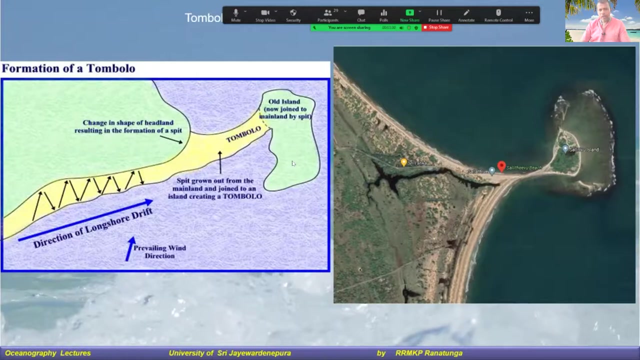 There is also a headland here. I don't know if you have been there. There is also a jungle beach. There is also a headland here. There are a lot of them. This is the island. I think you might not have heard about this thing called Thambolo. 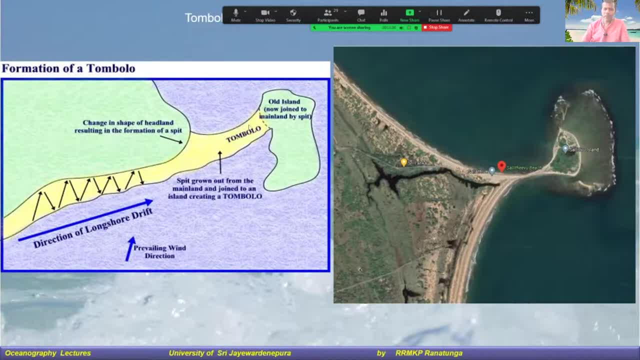 Thambolo is something you might have seen, but the term you might not have heard before. Thambolo is an island connecting to a mainland. This is an island. This is an island connecting to a mainland. It is a sandbar. 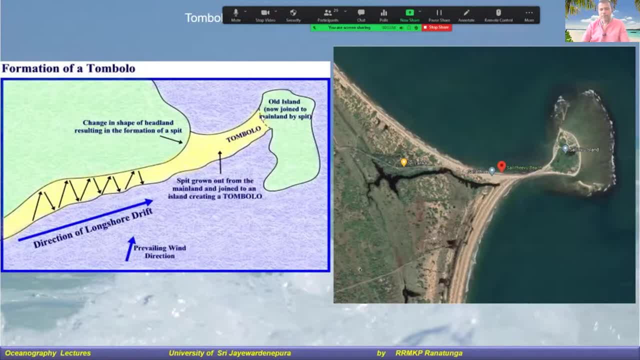 We call it Thambolo. This is a sand deposit. This is what it does. If you remember the longshore drift, there is a sediment here. This is how it works If there is a barrier on this island. this is a connection to the time of the Wadipura deposit. 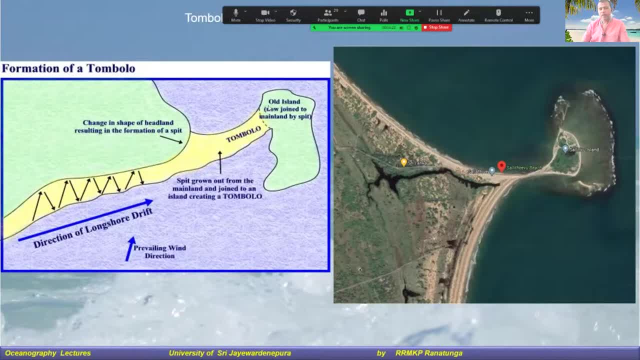 This is how it connects to that beach. This is how it connects to the beach during low tide They can even walk along this. That's Thambolo. This is an example of Thambolo island here in Xalithiu, If anyone from the east coast can enjoy. 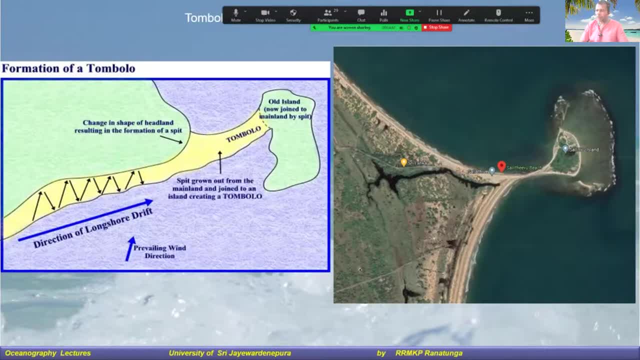 I should say met Urban Life in my town trip. I should say event in the east coast. If any of you have been to Haryam, you must have been to Haryam. If you have been to Kayankan, you must have been to Haryam. 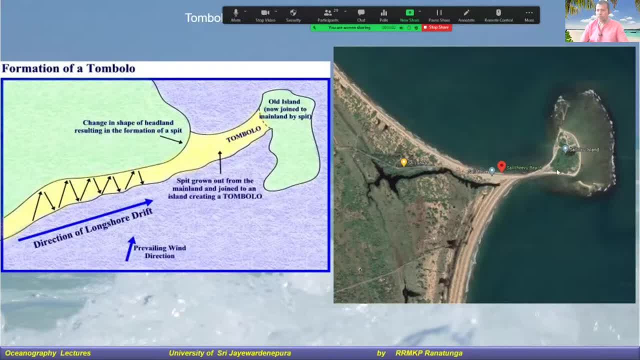 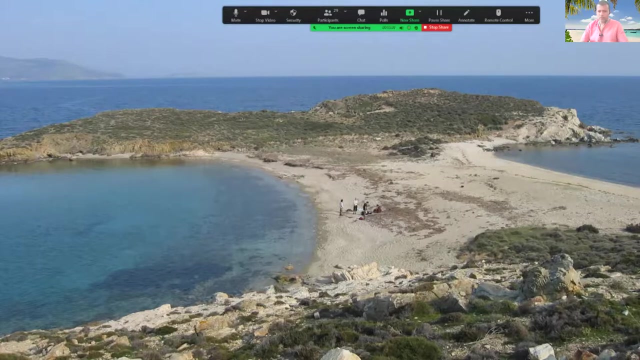 There is a small island here. There is a small island here. You can go there and see. You can go there and see. This is a good example from Sweden. This is not the Salithi Vaila. This is something from another country. 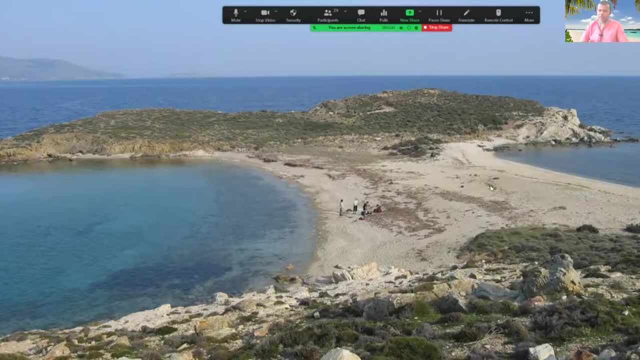 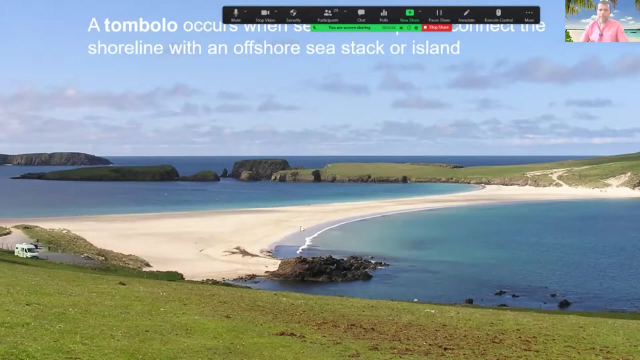 But this is actually what Thambolo is very meant. It can be like a permanently open island. It can be open sometimes. It can be inundated from time to time. It is connecting the two islands Like this. this is another country, Thambolo. 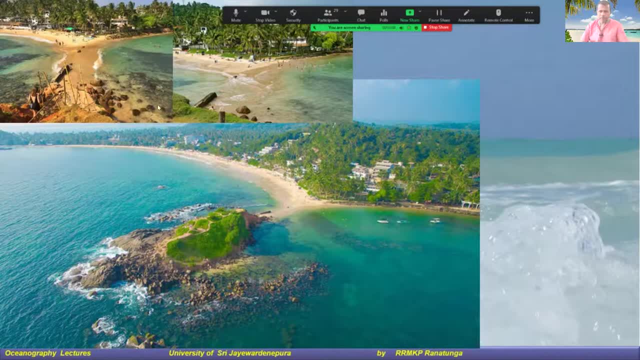 This is another example from Mirissa. I have taken it somewhere. This is Thambolo, And there is also one in Pomisen, But for some people this will stay at home In a underrule alone here. Right, You can start going somewhere in the Finnishpping dune weather. 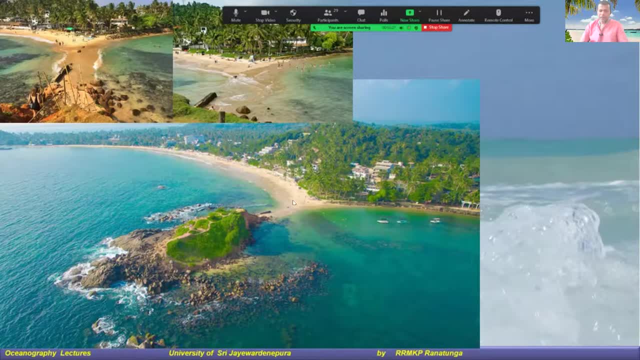 You cannot go where you want. You may leave and come Or go to Lothide- Just go there and do not stay too far away- Or travel, and also you may land in a wild place, A bit lost, But with continued care. 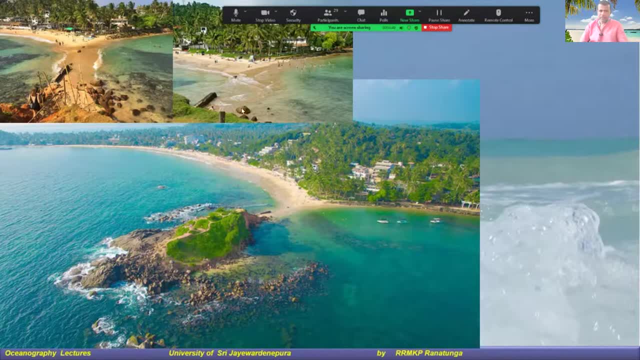 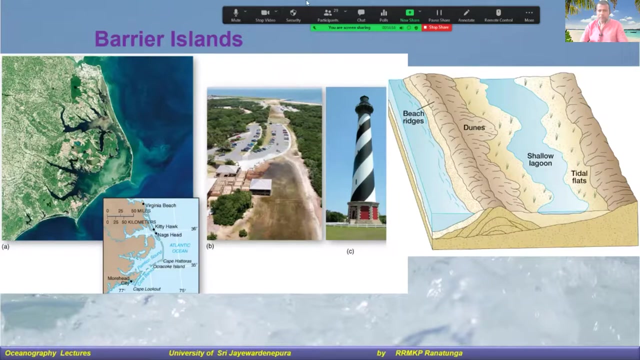 Without a doubt Very important. So make a movie, laughter, some pooling yet in the pool, and unless you're a good swimmer, So a lot of me, All right. So that's a tombola And, as I mentioned before, the barrier islands or the the same deposits islands are unique. 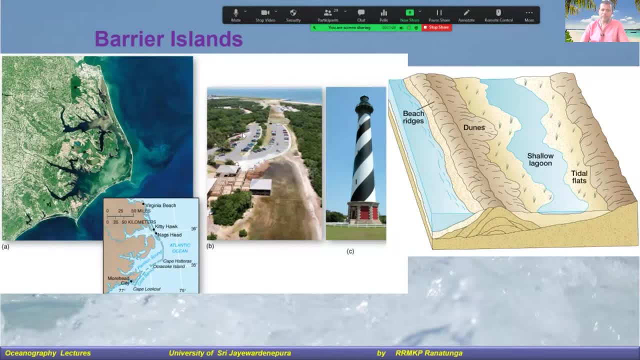 Type of a deposition of land, for you can see here, the island now has become A city with all their roads, and in Sri Lanka there are a few of these kind of islands, like in a Delph island. Nine of you, A way of being me. 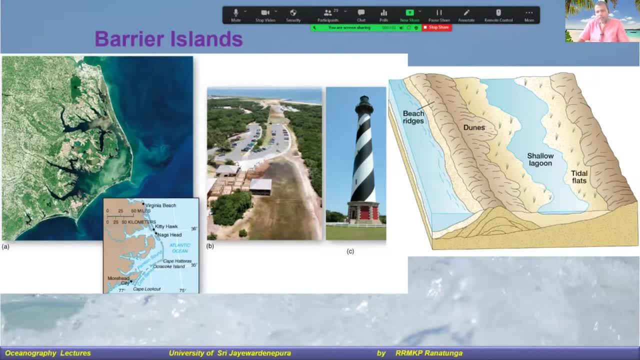 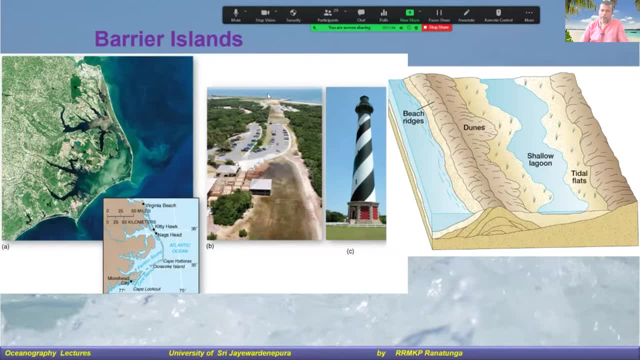 Of course we believe Otherwise. they're all actually islands, So they're all sand deposits. Very islands, Right? I was talking about the good You love under Delft to put up the way, And you are in the boat again. 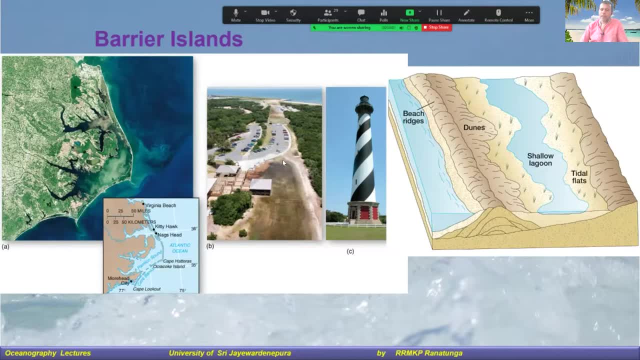 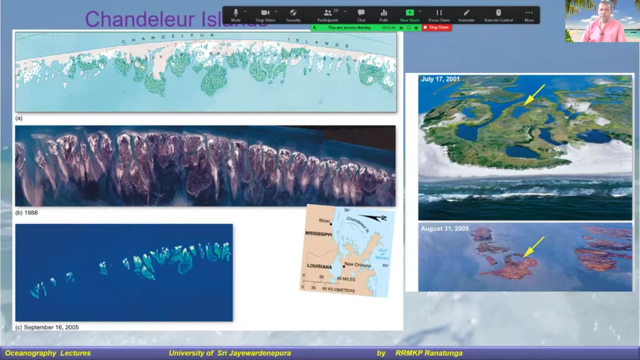 And then There's no any land connection. But once you go there it's just like a normal city, But it's an island Did there's no direct contact between the land. All right, all these are the barrier-built islands like sometimes can be island chains like this right.